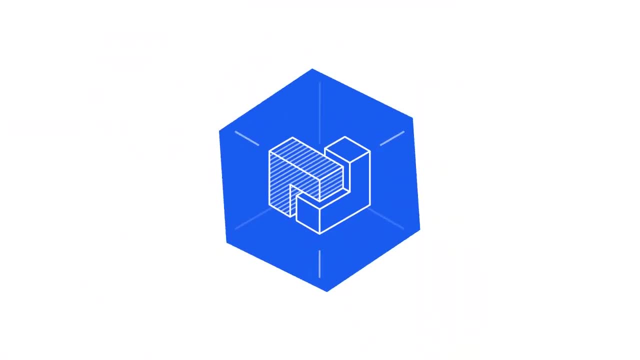 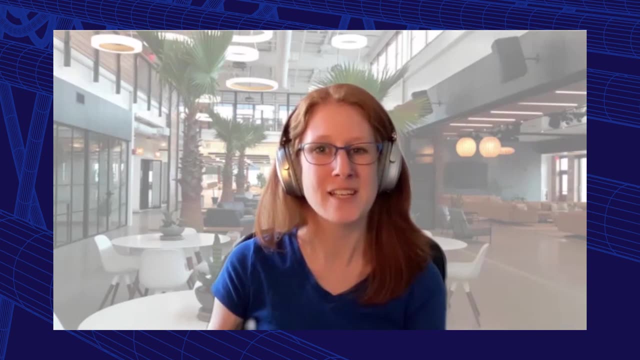 So, hey, everyone, welcome to today's Protocol Labs research seminar. Today we are joined by Alexander Viont, who's both a doctoral student and a research assistant at ETH Zurich. Alexander works with secure computational technologies, including FHEs or fully homomorphic encryptions. 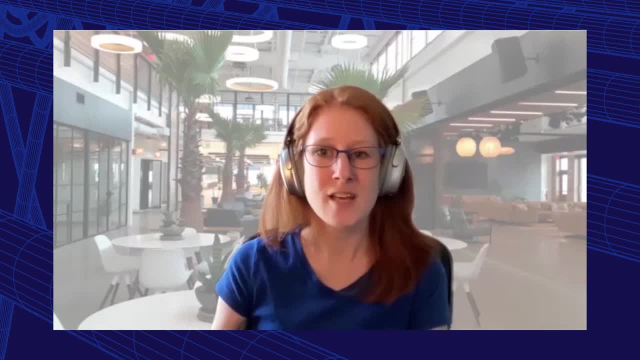 trying to make techniques more accessible to non-experts. Today, Alexander will be talking about HECO: automatic code optimizations for fully homomorphic encryptions. So, Alexander, I will let you take it from here. Cool, thank you for the introduction. So, yeah, hi, I'm Alex. 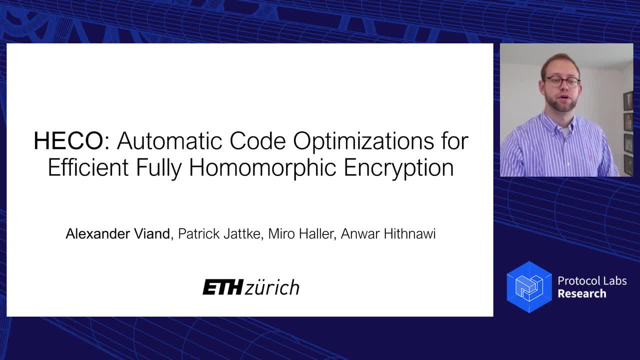 and today I'm going to talk a bit about our work on compiler designs for fully homomorphic encryption And, of course, as is usual with most of this research, it's work with a lot of collaborators, including some lovely students- Patrick Amiro at ETH- and also nice people like 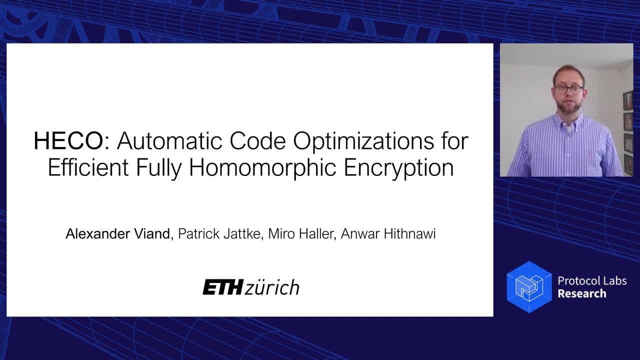 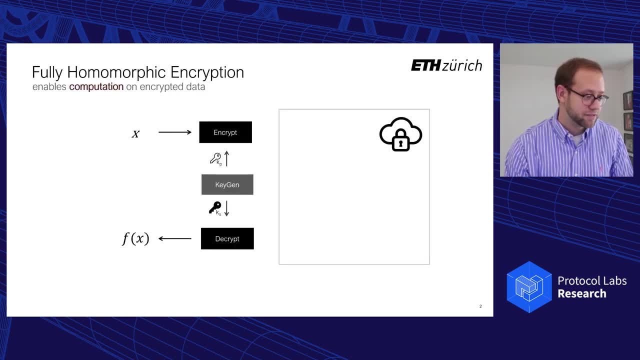 Amba. So what is fully homomorphic encryption? So what is FHE? FHE enables computation on encrypted data. Specifically, it allows us to delegate the processing of data to a third party without also having to give away access to the underlying data to that third party, And so that obviously has a 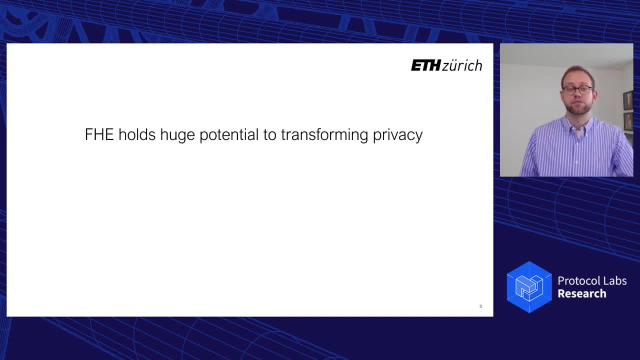 huge potential to transform privacy as we know it today, because it will, for example, enable us to provide end-to-end security for a much wider set of applications than what we can do today, And the good news is that, thanks to a series of dramatic performance, 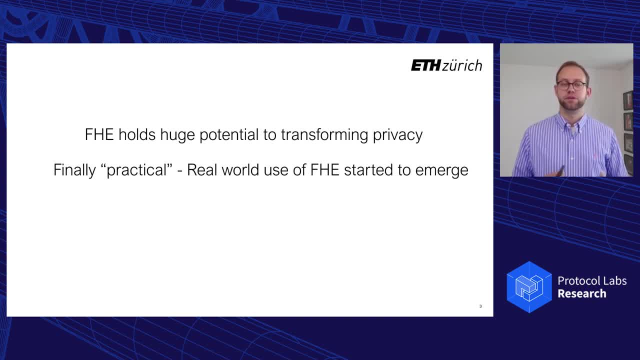 improvements. FHE is finally fast enough to be useful And, in fact, we're already starting to see it used in practice. For example, Microsoft has recently deployed fully homomorphic encryption as part of the Microsoft Edge Browser's password monitor service, which checks whether or not your 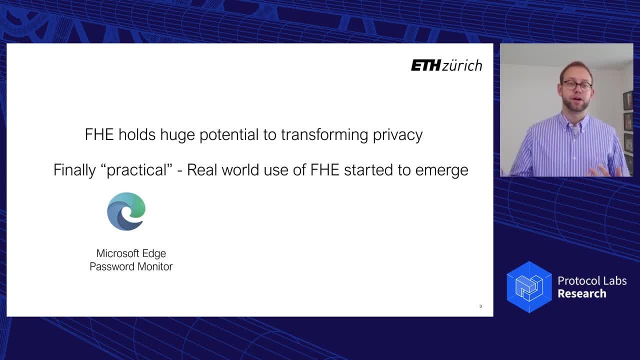 credentials are in place, And so it's a very, very important part of the process, And so we've been able to use that to operate FHE as a matter of fact, And so we've also seen some sort of perspectiva-like improvements, And so the clients experience will be much broader. 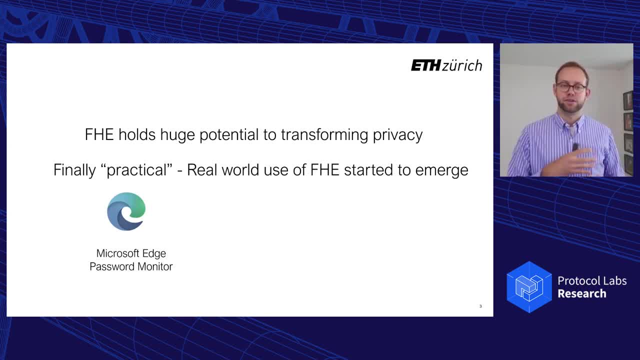 So there's such a large diversity in terms of the cake-and-touche features that Microsoft knows about. We've also seen smaller startups increasingly looking into how to commercialize FHE, mostly around the area of privacy-preserving machine learning, where you have a server that 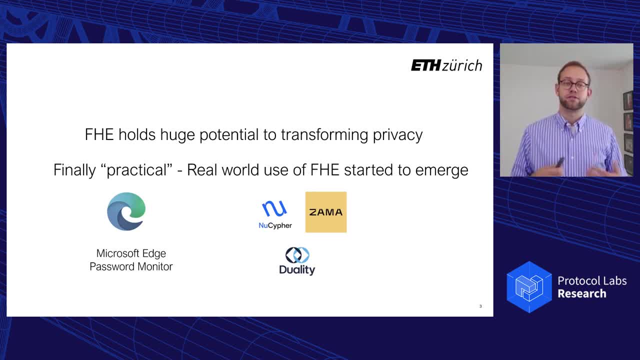 owns the machine learning model and you as a client can send an encrypted input and get back an encrypted transfer. So it's a change that we can make. So I don't know exactly how far FHE has gotten, but I think it's a fantastic piece of information. 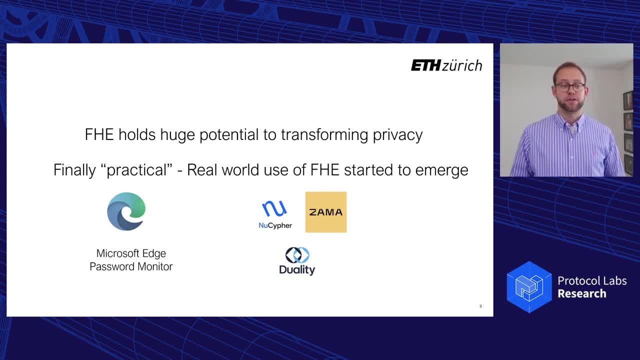 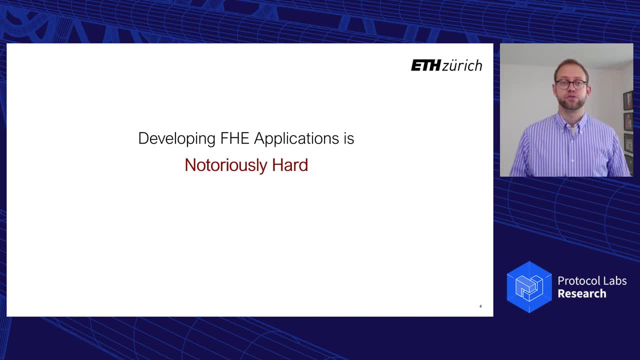 So we've also seen some smaller startups increasingly looking into how to commercialize inference results on that model. While there is a lot of promise in FHE, there is one big caveat, and that is that right now, developing FHE applications is notoriously hard. 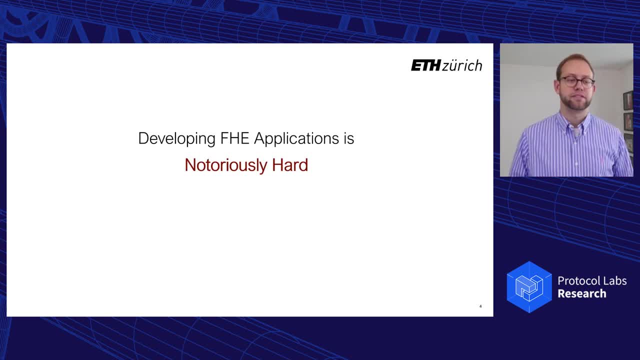 It just isn't generally usable yet And there's a lot of complexity in trying to make things work, And so for the moment, we're mostly seeing things like this password monitoring service being developed by a whole team of cryptographic experts. But of course, if you want to see wider use of this technology, then we must work on making 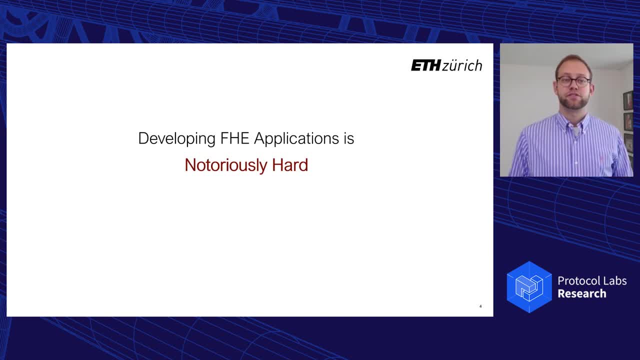 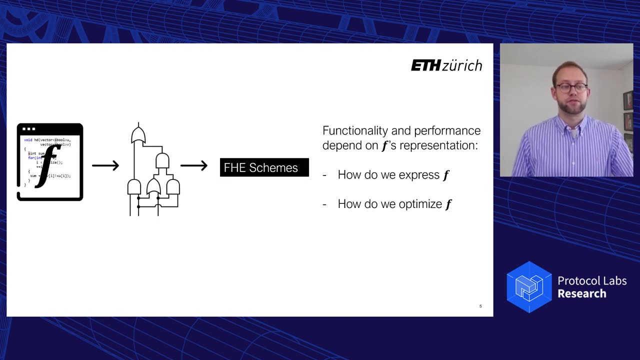 it more accessible, And so today, I want to briefly touch on what exactly it is that makes developing FHE applications so hard, and then go into how compilers and tools like compilers can help to address these complexities. The reason why it is so complex to write FHE applications is that good performance tends 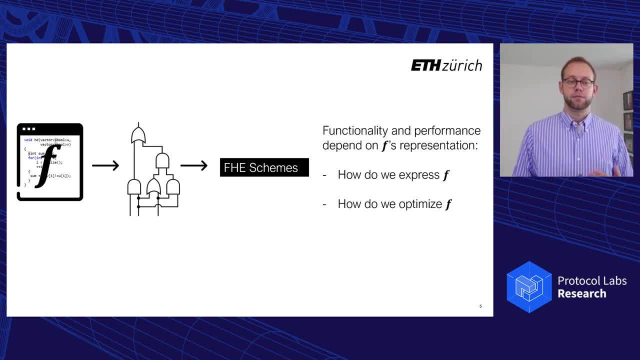 to require fairly extreme performance. So how we express our programs and how we optimize them is kind of crucial for good performance. The sort of trivial, straightforward implementations in general will be exceedingly slow in the context of FHE And even fairly small changes in the application can result in drastic differences in how you 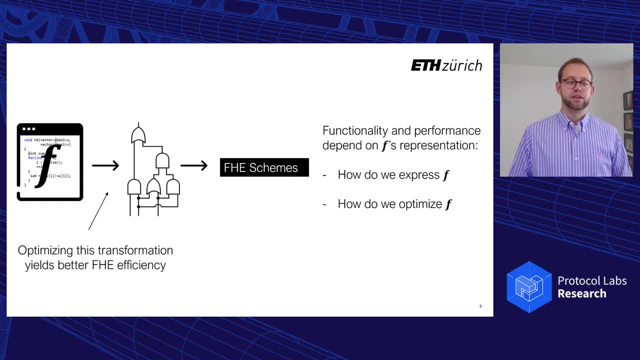 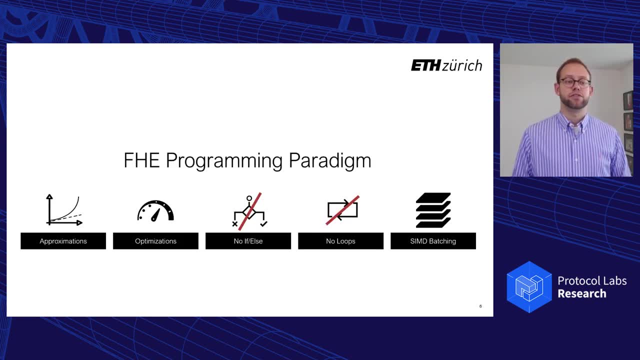 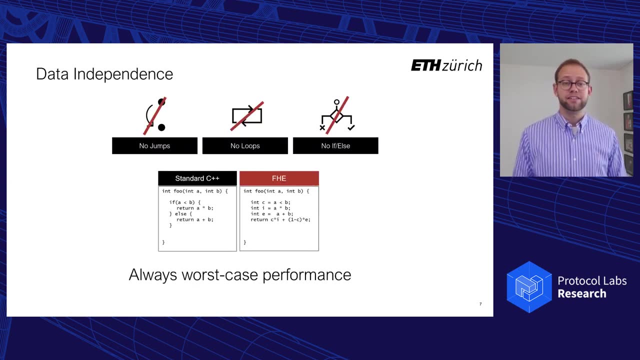 should implement it and then how well it will run right. And so FHE imposes a lot of constraints And that in turn then results in a fairly unique programming paradigm for FHE. As an example, data independence is sort of built into FHE because, by definition, computations 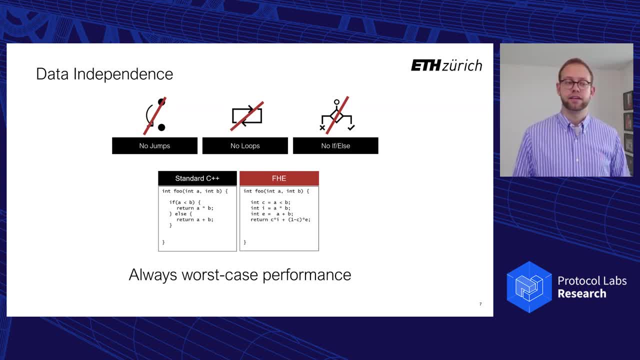 in FHE are a black box from which no information must leak, And that includes things like bits about whether or not we branch, And so we cannot do data-dependent branching. That means no jumping, No dynamic loops And not even real if-else statements. 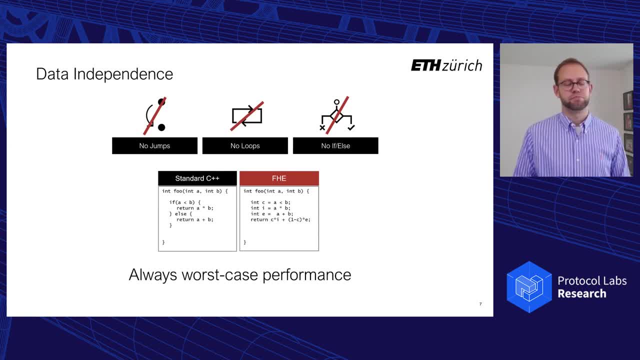 We actually can emulate things like if-else statements by doing this multiplexing-like thing that you can see here on the slide, But note that when we do that, we actually have to evaluate both sides of the branch right, And so, in general, data independence means that the runtime of your sort of secure computation 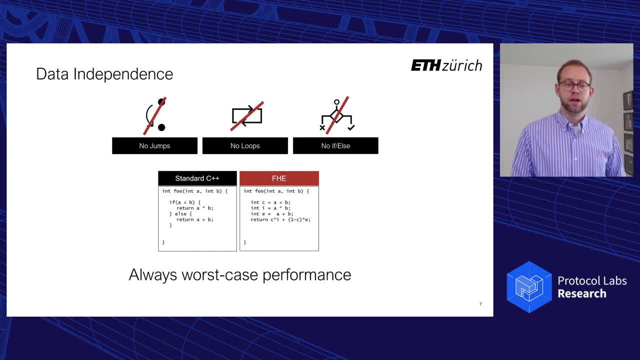 is always at least the worst-case runtime of the original algorithm, But in practice it's always the worst-case runtime of the original algorithm. But in practice it's always the worst-case runtime of the original algorithm, But in practice it's frequently much, much worse, even before you consider the actual 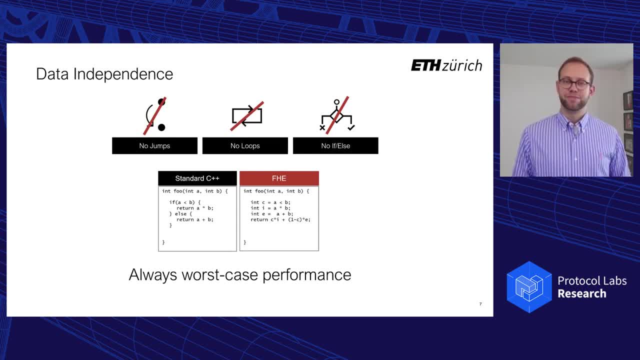 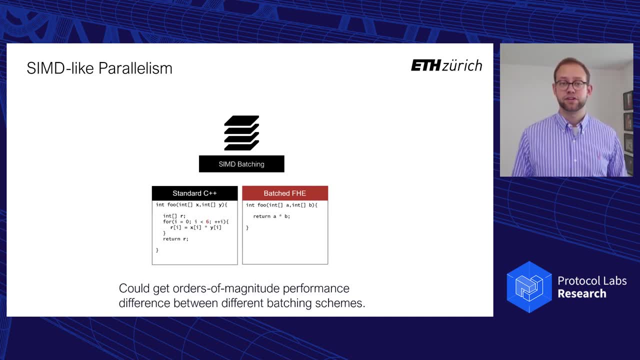 overhead from doing the crypto and the math. Obviously, that's maybe not the greatest news, but there is good news as well. in the world of FHE, For example, a lot of the major FHE things right now offer a very powerful but restricted 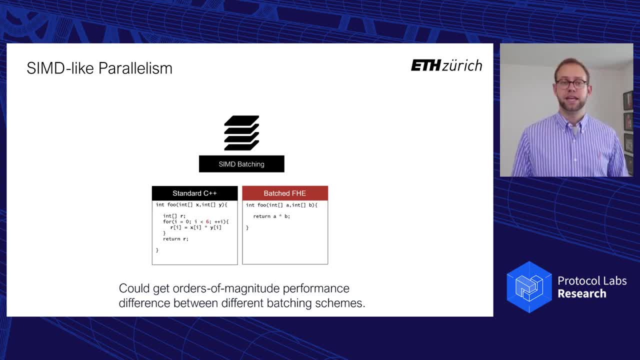 form of data parallelism, So you can encode many thousands of integers into a single ciphertext rather than just a single one, and then operate on them in a single instruction. multiple data: Yeah, And it's really really fast and very efficient. You can run it in a single function in a single time fashion. 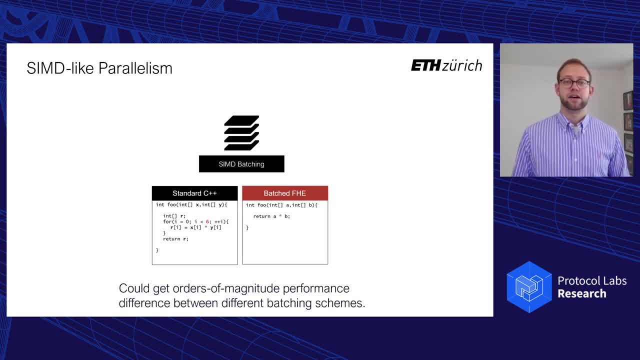 That can obviously give you a massive amount of speedup, but the catch is that you're very limited in terms of data movement, So you cannot sort of treat this like an ABX type form vector interaction. It's much, much more restricted. 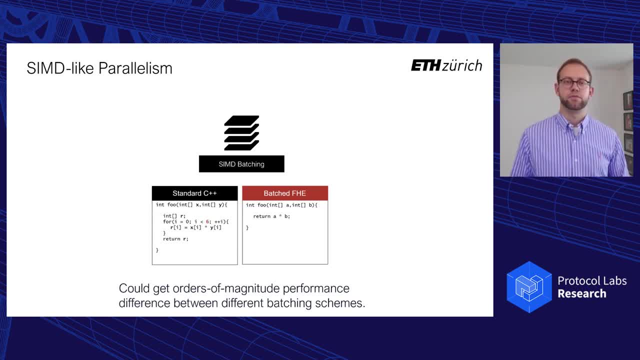 And so using this in order to enable actual improvements in the latency of applications rather than just sort of paralyzing and improving throughput, is actually a fairly significant challenge. But it's worth tackling this challenge because doing so tends to give you several orders of magnitude in speedup, So it's not unusual to 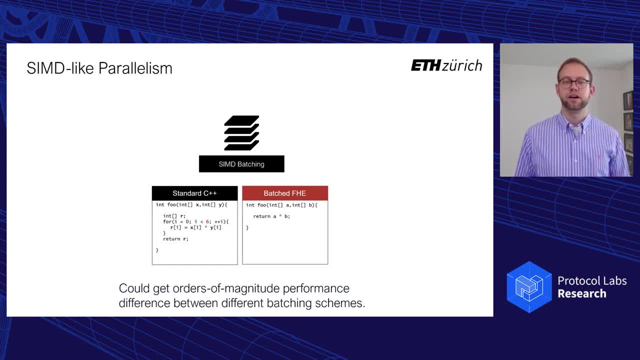 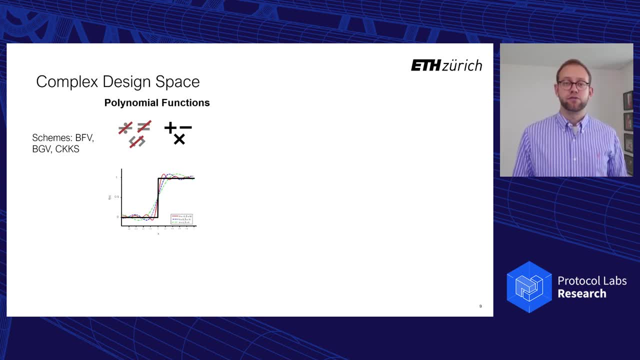 see 10x, 100x or even higher amounts of speedup from applying SIMD parallelism to a problem, And of course I'm only touching on a few highlights here. In general, the FHE design space is relatively complex. For example, most of the schemes only natively. 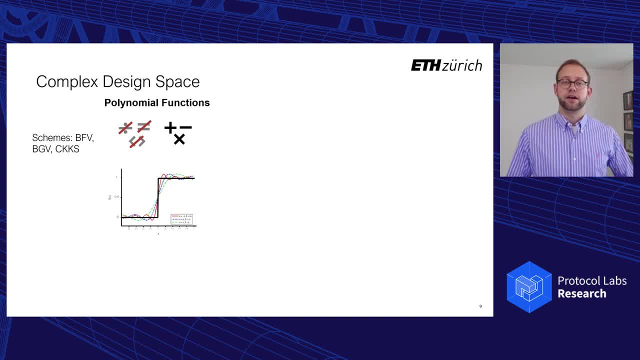 support additions and multiplications, And while that obviously allows you to compute any polynomial function of the integers, that isn't necessarily the kind of things you want to compute, And so you can use polynomial approximation to sort of get around that. But it turns out that in practice, with the restrictions of epigee, it's very hard to find. 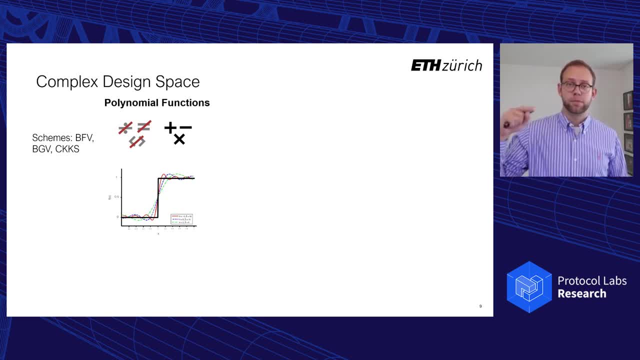 the balance between the accuracy in your polynomial approximation and the performance of that approximation. And so, alternatively, if you need non-polynomial evaluation, you can look to the FHE design space. And so, if you need non-polynomial evaluation, you can look to the. 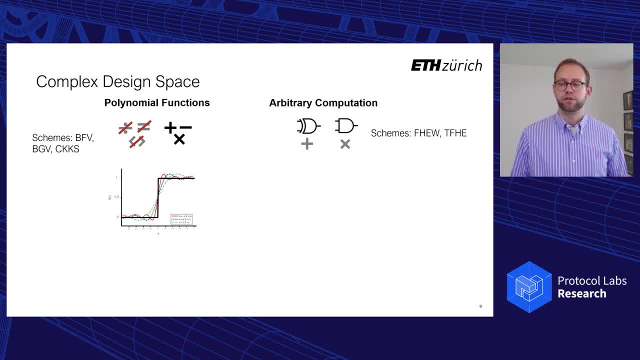 FHE design space, And so if you need non-polynomial evaluation, you can look to the emulating binary circuits. So if you imagine addition and multiplication in Z2, well, that's just X4 and AND, And so with that you can do arbitrary computation. But the catch is that now 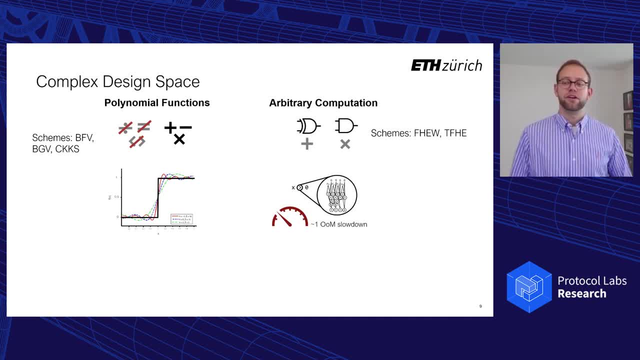 every single operation in your input program is getting turned into dozens, if not hundreds, of actual epigee operations that compose these, let's say, binary adders, binary multiplier circuits that you are now having to emulate. So, at the very least, 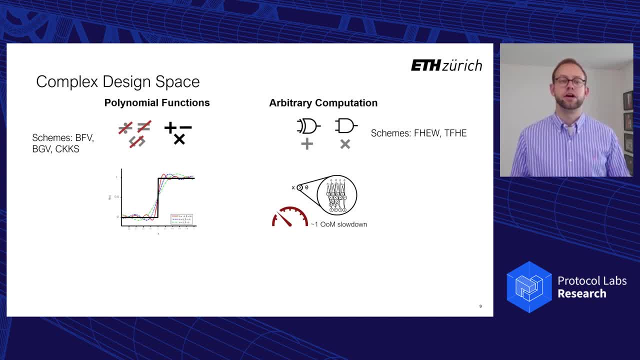 when you're using this approach, you're seeing about an order of magnitude slowdown compared to doing things directly over integers, And in practice it tends to be much worse, actually, because of sort of compounding factors. If that wasn't enough, then you also pretty much always 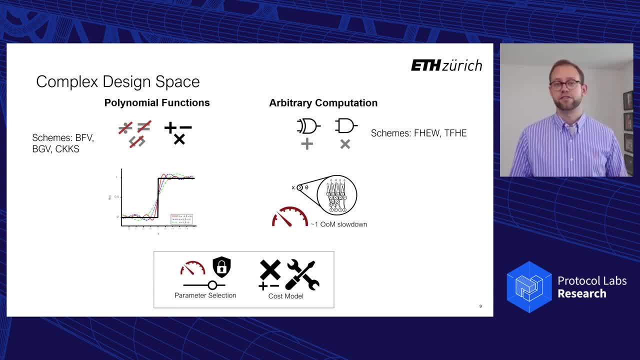 in both of these settings have to consider things like parameter selection. This requires balancing security, performance and accuracy, And so it's not just a thing of looking up the standard. It's really per application. you need to figure out what are the correct parameters. 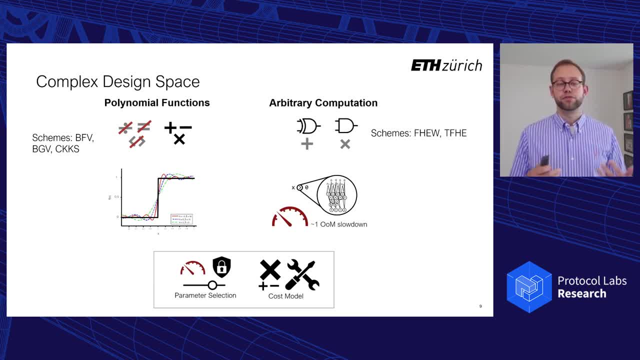 for this specific task And you also have to deal with this very unique cost model of FHE. It's somewhat like MPC in that additions are much cheaper than multiplications, But in fact in FHE most of the runtimes are dominated by these scheme-specific operations. 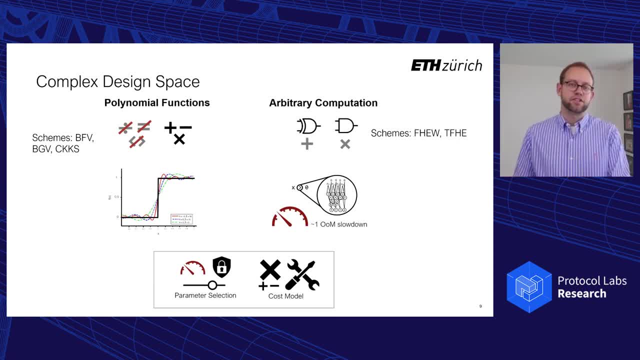 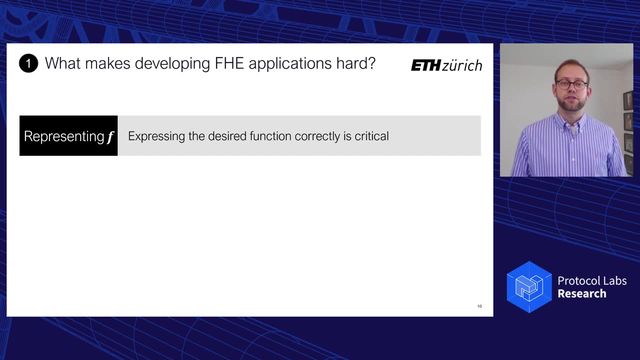 that don't actually modify the message on an application-level object, but they're just required to maintain the cytotext as the computation goes on, And so this is also something that you just have to wrap your head around. In summary, developing FHE applications is hard because it requires looking beyond the overhead. 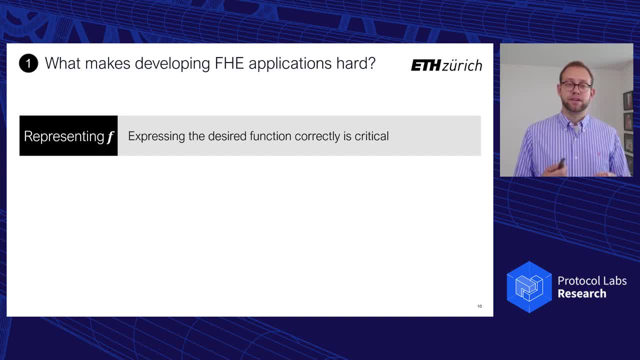 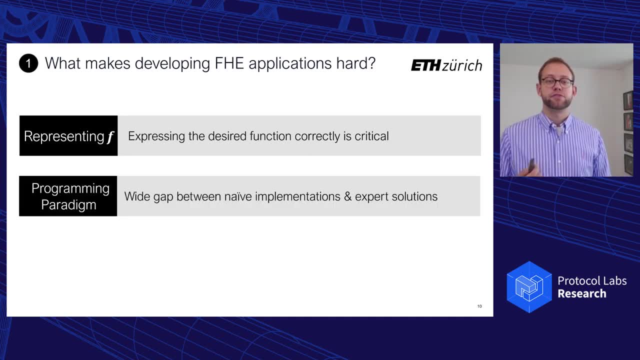 of the underlying FHE operations And really the application design has a significant impact on the performance, And so you need to spend a lot of time on that. As a result of that, we see a massive performance gap between sort of naive implementations done by non-experts. 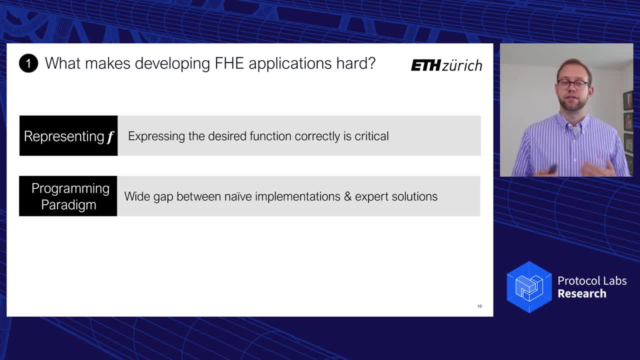 and first-time users, and those that were carefully designed and fine-tuned by experts with maybe a PhD or even a faculty position in this field, And so the design space obviously is very complex. There's a variety of different approaches. 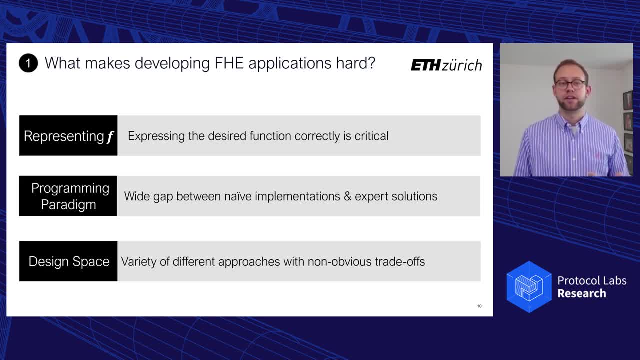 and they all have non-obvious trade-offs, so that even for experts it's not even entirely clear what would be the best approach for every problem. But for non-experts it's usually completely and transparent where to even begin with your implementation. As I said, I want to keep it. 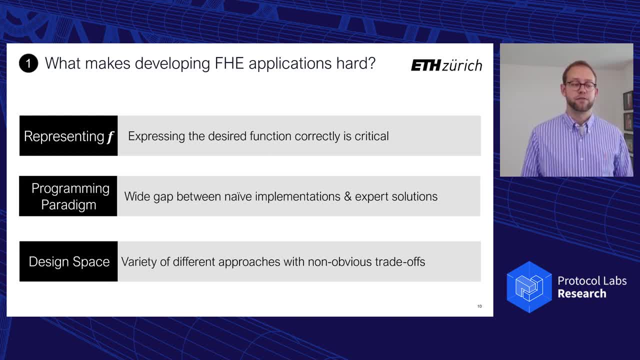 fairly brief on the challenges that we're going to be dealing with in the future. So I'm going to go into a little bit more detail about the challenges today, because we actually have a paper about this from last year where we go into a lot of the detail, a lot more detail about 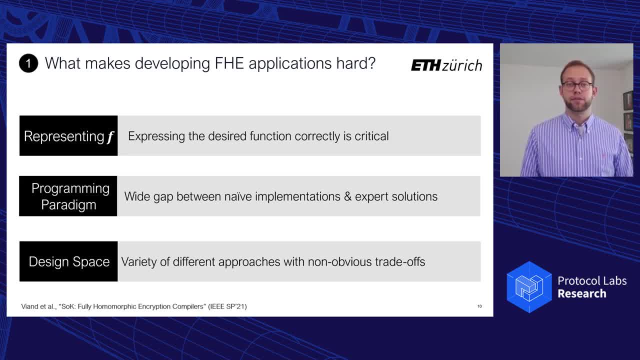 the challenges and what it means for sort of everyday developers. If you're interested in learning more about that, you can either check out the paper I linked below or we also have a talk about this recorded that's available on FHEorg in the list of previous talks there. 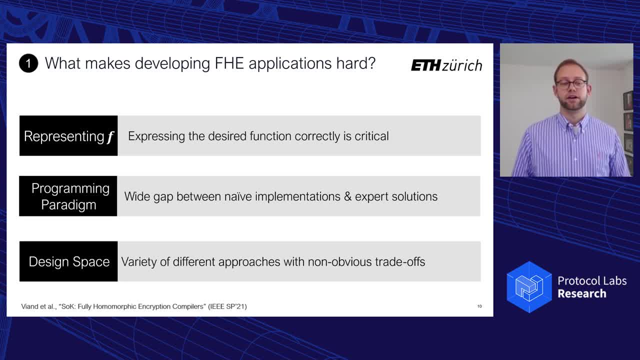 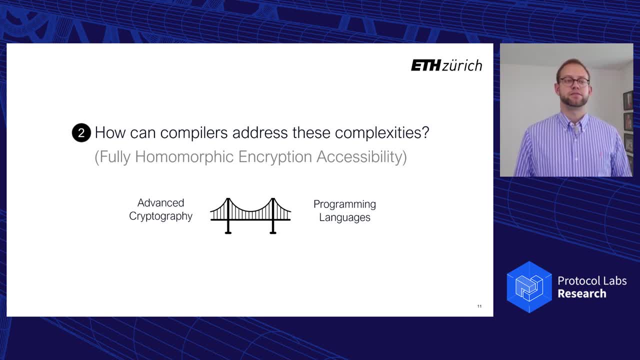 So yeah, but today I want to focus on that and instead I really want to focus this talk on asking what does help in addressing these complexities? And that basically means asking ourselves how can we make FHE accessible to non-experts, And we propose that that requires combining concepts. 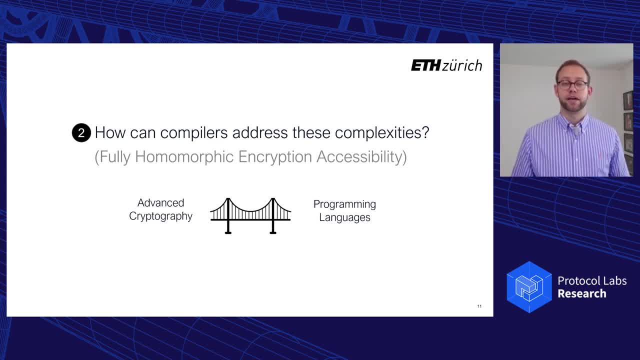 from the crypto side from the other one hand, and then programming language design, in order to be able to bridge that gap and to develop tools and abstractions that facilitate FHE development. And I personally happen to believe that compilers are the key to democratizing FHE. 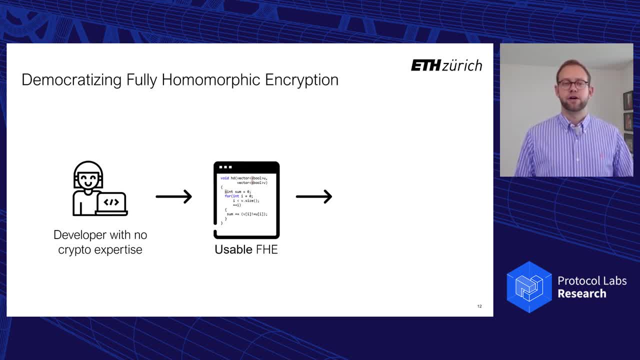 Because delivering on the promise of FHE requires tools that allows non-experts to actually develop. you know, turn the existing code into efficient FHE solutions with ideally minimal changes, And in that world the compiler should be taking care of most of the complexity. 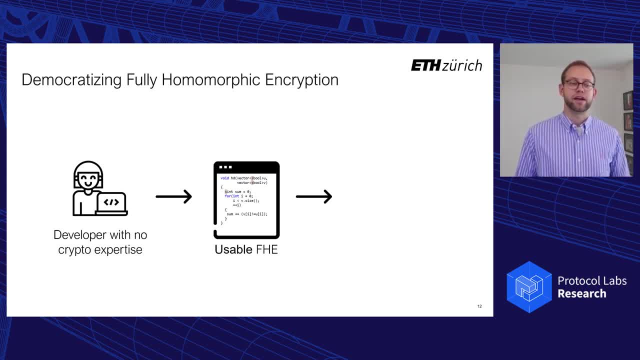 allowing the developers to express their computation tasks that they have in a high-level language, and then the compiler automatically generates and optimizes secure and efficient FHE code. from that And towards this vision, we have focused primarily on two challenges in our research. 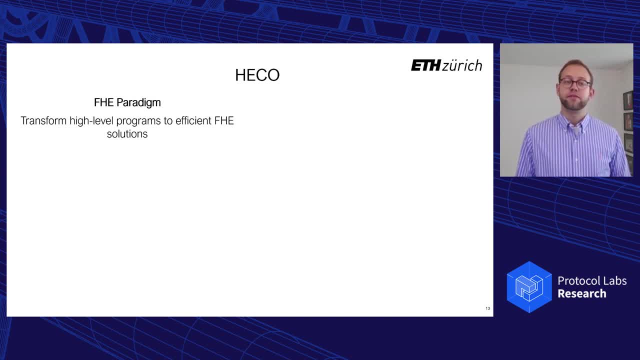 The first one is automatic translations. Specifically, we're focusing on mapping high-level imperative codes, which doesn't really mesh well with the programming paradigm of FHE. And how do we map that to efficient batch FHE solutions automatically without requiring user input? Well, minimal user input. for example, we do require the user to annotate which values the 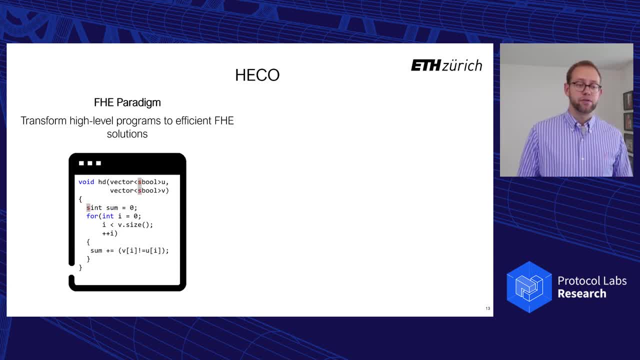 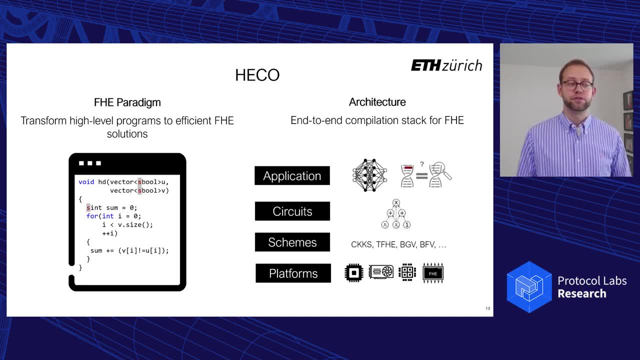 FHE code is, So we need to make sure that we're actually mapping the FHE code in the right way. On the other hand, we're also bringing in a new architecture for FHE compilers that we believe much better reflects the different optimization opportunities. 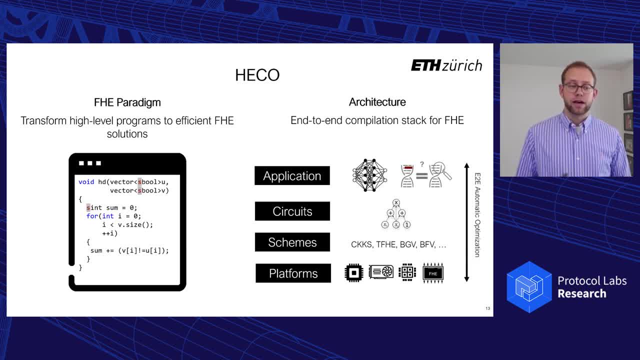 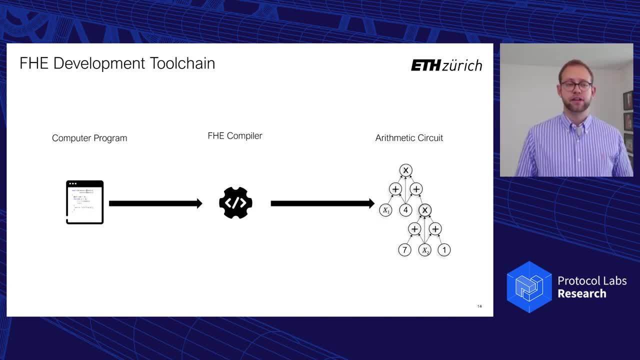 that the FHE stack allows for, And so I want to have a closer look at what we actually mean by an end-to-end development tool chain for FHE. Traditionally, we might think of an FHE compiler- and this was definitely true, let's say, two, three years ago- as a tool that converts a program in 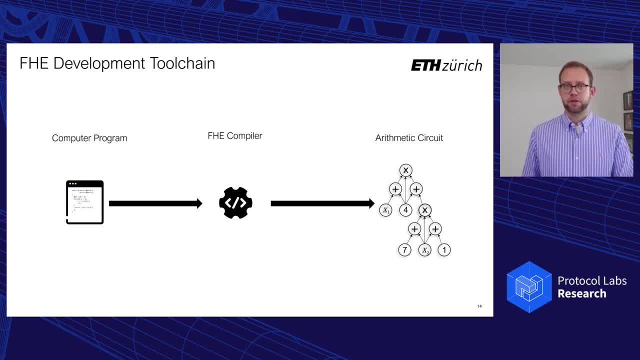 some more or less high-level language into an arithmetic circuit, And the arithmetic circuit is sort of the natural and traditional mathematical model of an FHE computation. If you then want to have an optimizing compiler, well, that means probably rewrites and simplifications on the circuit happening before you put it around, But in reality we see that FHE 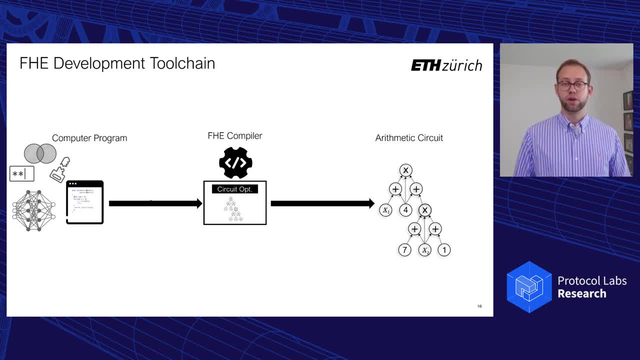 applications come from a whole range of domains, which all have different paradigms used to express the programs, And so when we directly translate these various high-level paradigms into circuits, what happens is that we lose a significant amount of information, and making it much. 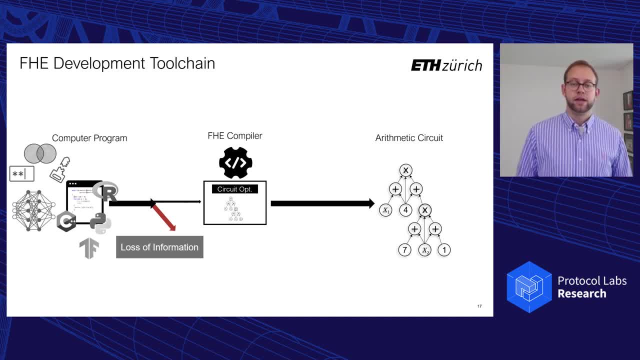 much harder to actually work with and optimize the program, And so one of the first things we do is we propose to extend the notion of an FHE compiler sort of outwards towards the front end, by introducing program optimizations that make use of the high-level information that is present in the 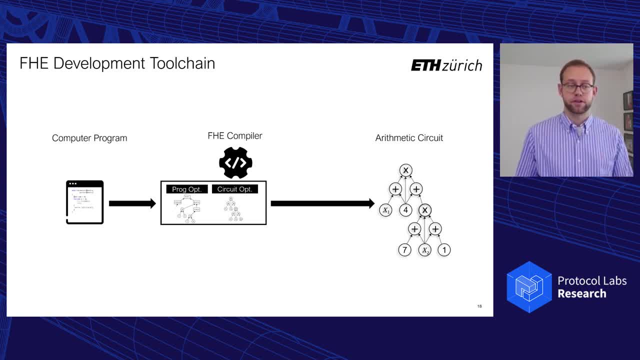 input program, while it's still a program and not a circuit. And on the other end of the system, we acknowledge that really what the end user wants is not an arithmetic circuit. What they want is instead a secure and efficient FHE implementation right. 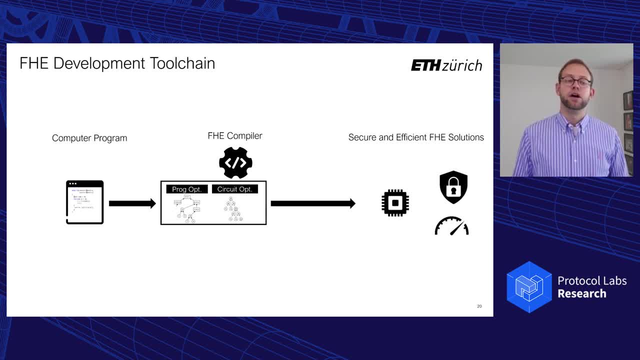 And so that can mean having an executable that works on CPU, but also increasing the GPUs, FPGAs. we've seen work for that in FHE And then, in looking towards the future, FHE's specific ASIC accelerators that are currently being developed as part of the DARPA DEPREC program. 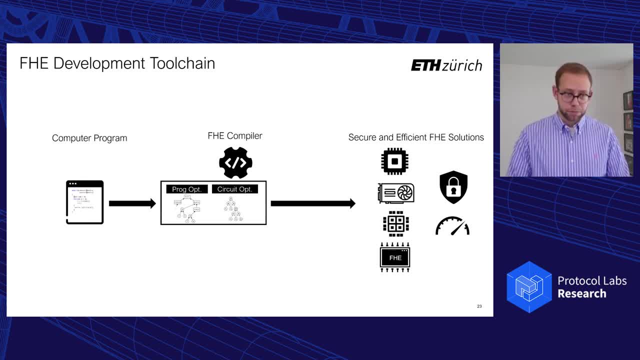 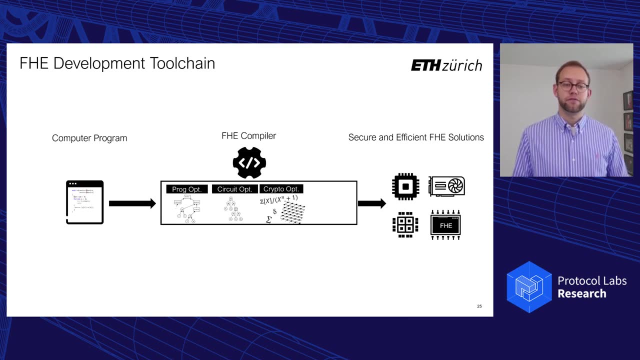 by a couple of competitors, including, for example, Intel. So in order to support all of this, we also need to extend the compiler on the other side. so to the right here, with the ability to target hardware first by lowering FHE operations to the 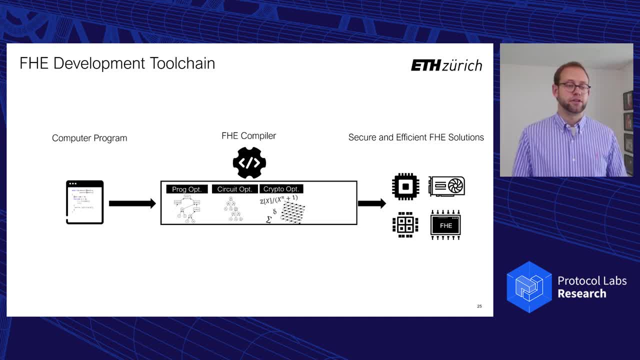 underlying map and then going further and scheduling these low-level operations appropriately. So that is sort of the zoomed-out view of what we think an end-to-end FHE development toolchain needs to be. So how do we actually go about building such a compiler? 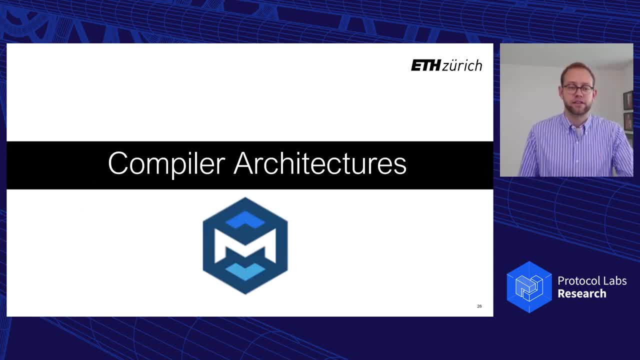 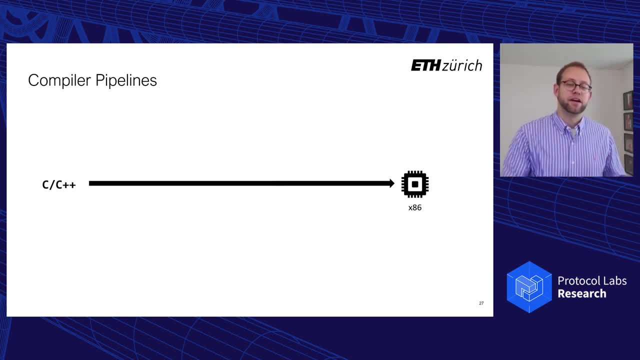 And for that I want to take a very brief look at the evolution of compiler architectures. So the traditional compiler is this monolithic tool that takes in, let's say, C or C++, and then, through a number of transformations, crunches it down into assembly for a specific 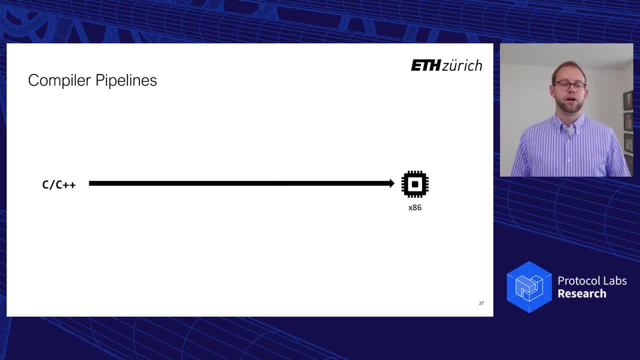 target, And this is basically the architecture of GCC. But we soon realize that there are significant advantages to introducing additional intermediate representations, like the LLVM IR that is used to enable the Clang compiler to retarget to a variety of different backends from the same starting point, And this means that each of the translation steps that they now have. 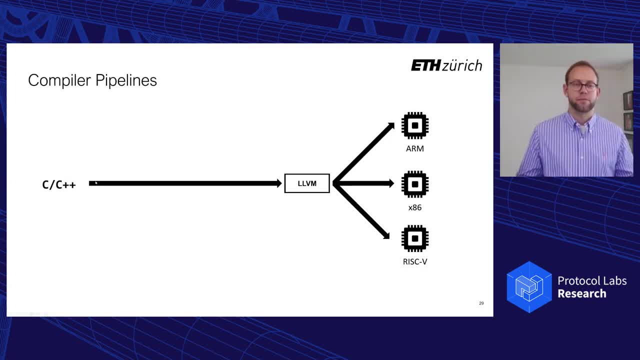 to do is significantly smaller than the sort of large gap that something like GCC has to cross. But it turns out that for high-level language, especially higher-level languages than C, C++, this is still a pretty large gap, And so we see compilers for Swift, for example, introduce. 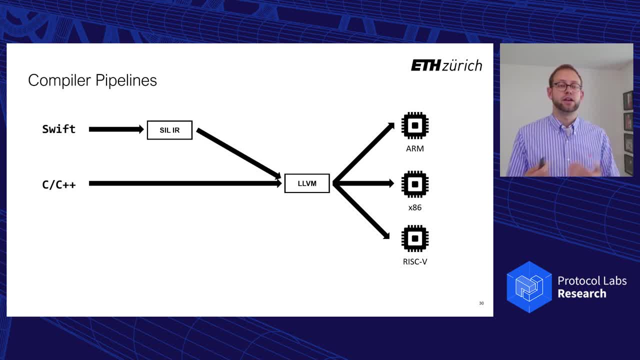 their own high-level intermediate representations, but then lower, for example to LLVM, And we're seeing this trend towards an increasing number of abstraction levels. For example, with Rust, we're now seeing a high-level and a medium-level intermediate representation. 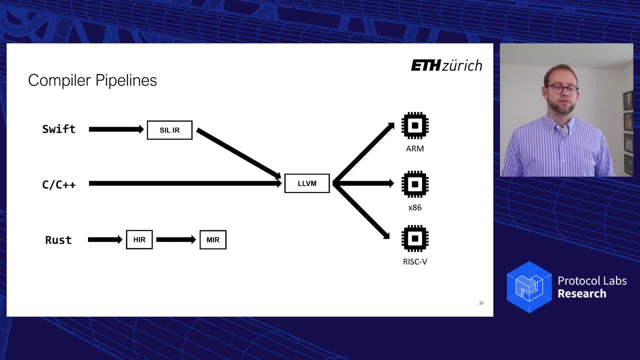 before they're targeting LLVM, And this trend really goes to its conclusion, sorry, with domain-specific languages. So with domain-specific languages we have a large number of intermediate representations and that means that the individual loading steps between them are much, much easier to express, to the point where you can sort of fairly easily express: 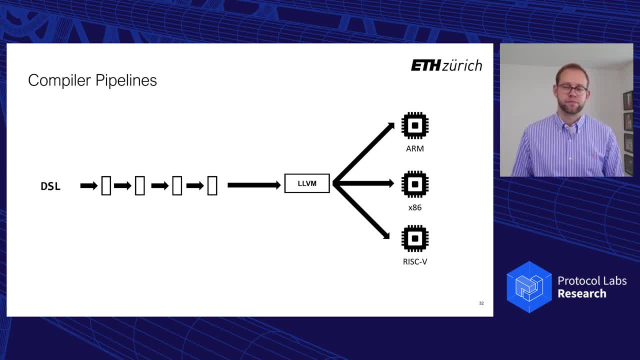 them as a domain expert rather than as a compiler expert, And so this is exactly what we're also using for our compiler Eco, which is a homomorphic decryption compiler- Sorry, we don't have the most creative acronym there- And in our case this looks like this, right? So? 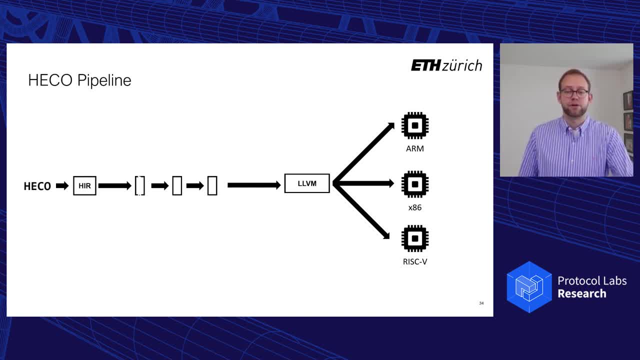 from the input program we first go into a high-level intermediate representation and here we still have our control flow, our high-level operations, like linear algebra operations, right, So even higher level potentially than C. This is then lowered into this, eventually, autism optimization into scheme-specific intermediate representation. 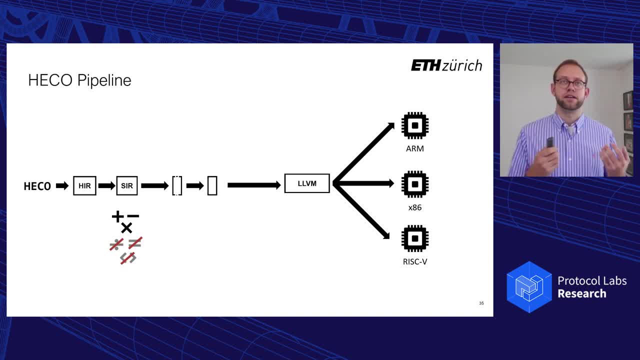 and this is basically sort of representing the native operations of an FHC scheme. Most importantly, this means not having all of these convenient functions like equality, comparison etc that have been sort of stuck in this multiply and etc world. And then when we 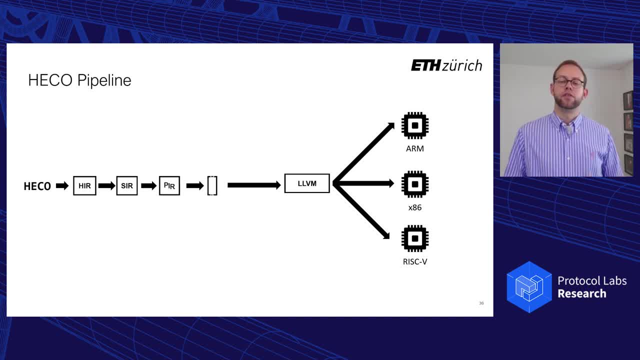 want to go lower and actually target hardware, well then, which translates to the polynomial intermediate representation, which actually is there to represent the underlying map of these schemes. And then there's another step, which is the RNS, or residue number system- intermediate representation, which is representing an abstraction of how to efficiently work with. 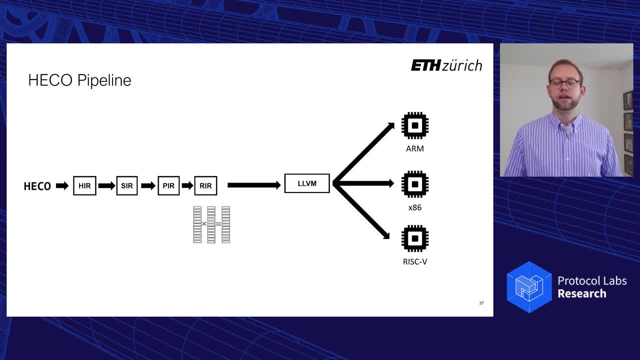 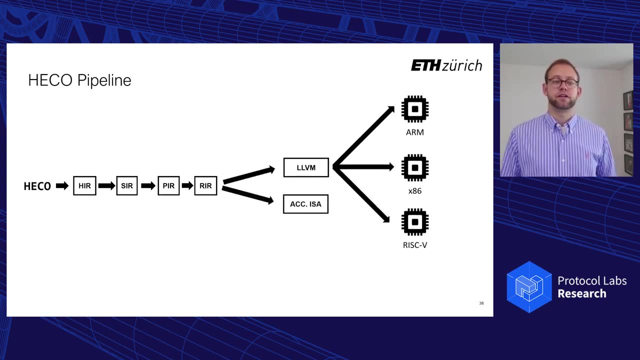 large-degree polynomials and large-big-width polynomials in sort of fixed-width hardware. So all of these obviously are designed to translate and lower down to LLVM and then inherit from that the existing targets. But we also envision that in the future Eco will target the ISA or instruction set architecture. 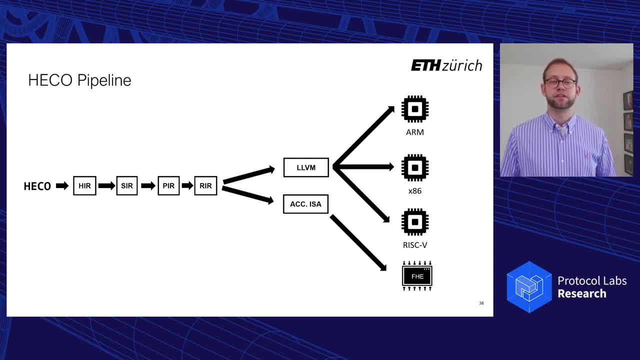 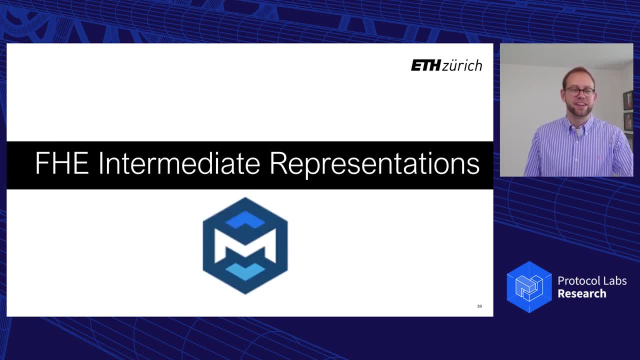 of these upcoming data-deprived accelerators specifically built for FHC. I think I've said the word intermediate representation a whole bunch in the last minute or so, but let's actually look at what is an intermediate representation And specifically I'm saying this in the context of 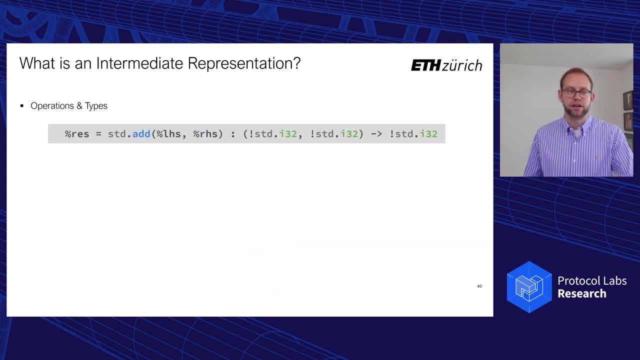 the MLIR compiler framework, which is what we're using to realize Eco. So here an intermediate representation is basically a description of, let's say, an API. You have an operation that belongs to a dialect so standardadd, It has operands, It has results, It also has types- Very important. 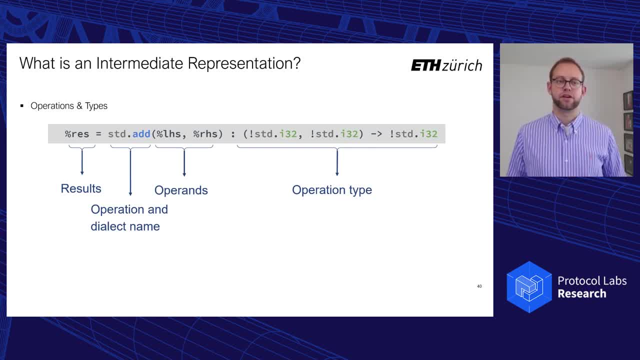 for the actual implementation of things, but I'm going to completely ignore that for this presentation. And then this basically defines the syntax in some sense of your intermediate representation. But whether or not this actually means anything isn't defined here. right, We can. 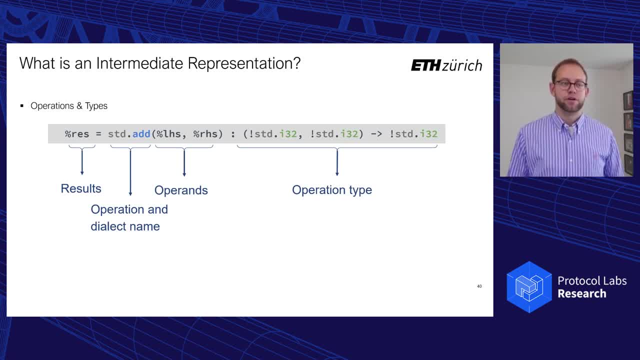 expect that standardadd probably adds to numbers, but this actually isn't defined as part of this. It's defined through lowering. So it's not defined as part of this. It's defined through lowering. So, to give you a bit more of an interesting example, that isn't just an addition. So let's have a look. 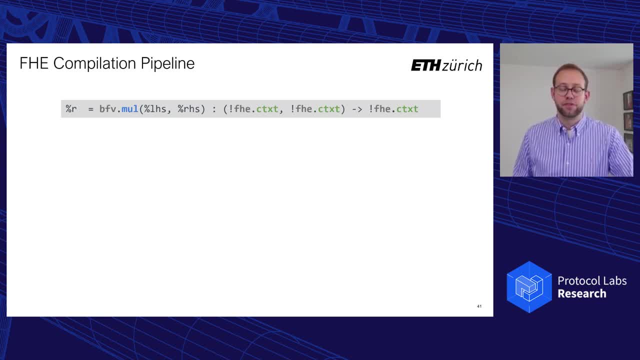 at the VFB multiplication operation. So this is quite a bit less trivial than, let's say, an integer multiplication, because it translates to first of all a series of polynomial multiplications between the polynomial elements of the ciphertext, And then actually each of these polynomial 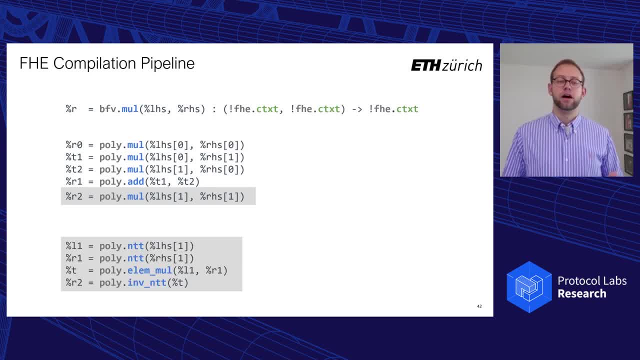 multiplications translates even further into, let's say, an entity or element-wise multiplication, then inverse entity, which is a way of performing large-degree polynomial multiplications efficiently. In fact, each one of those would actually translate even further into the RNS level IR. 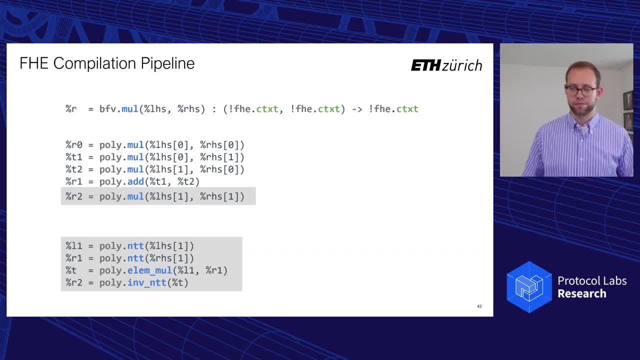 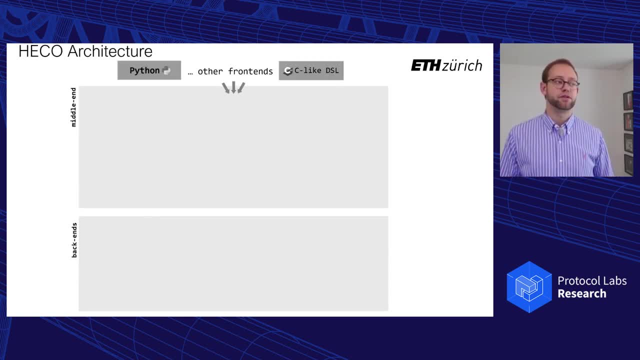 but that gets way too verbose for this overview. I've zoomed in here a bit, so let's zoom out a bit. Let's have a look at what's actually happening here in terms of architecture. We have a Python front-end and we also have currently a C-like sort of domain-specific. 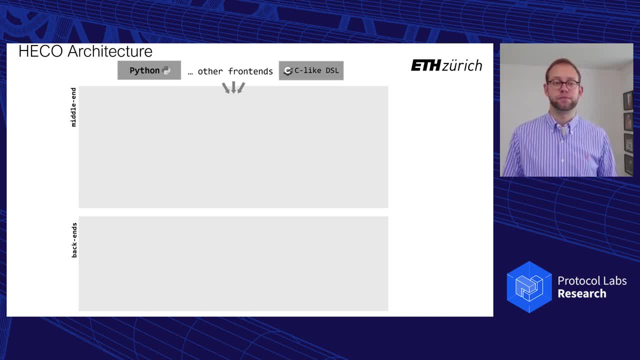 language front-end and we're very open to adding more front-ends if people can sort of show us why they would prefer one. All of these front-ends, they translate the input program into our high-level intermediate representation. This is made up of our custom dialect or set of operations around FHE. 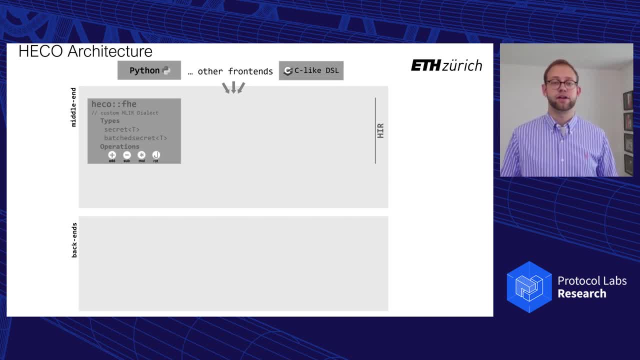 but it also includes- and this is an advantage of using something like the MLIR framework- built-in dialects and operations like the tensor or vector dialect, ones for basic arithmetic, for control flow in terms of define, function calls and all of these things that we get to. 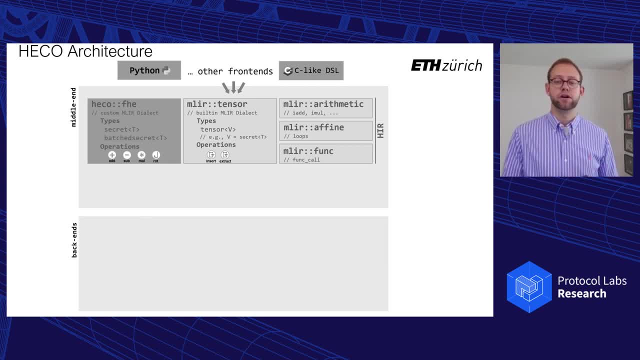 inherit. By cleverly connecting our FHE dialect with the built-in systems, we actually get to benefit from a lot of the built-in optimizations and we basically avoid reinventing the wheel for some of the compiler 101 stuff. As I said and just showed earlier, this then gets translated to scheme-specific IR, For example. 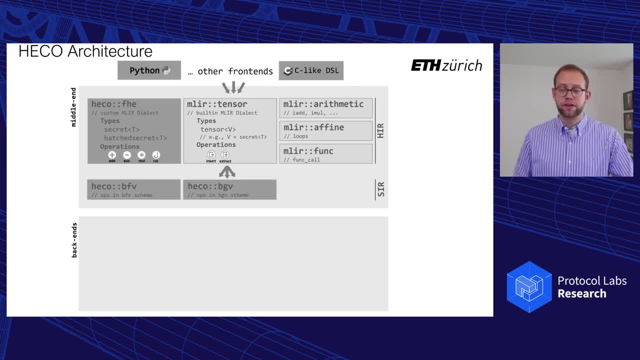 this bfbmult operation that I just showed is from this BFB dialect, and then we have dialects currently called BFB, BGD and CKKS, which are the ring-based FHE schemes that will have this SIMD ability that I mentioned earlier. When we then want to translate that into an actual 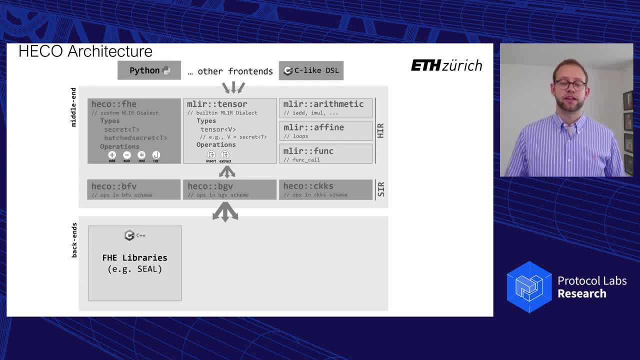 computation. the easiest way would be to just translate it into calls into an FHE library like seal, which implements all of the crypto by itself. But increasingly we're seeing that there's interest and demand for being able to actually lower to hardware directly, and this 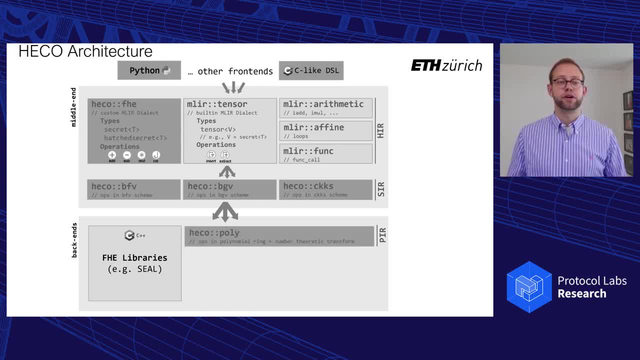 is then when we do what we just saw, which is lower into polynomial operations, Those- and that was the thing that didn't fit on the slides- get lowered into RNS- Residue Number System- operations, and then, finally, this gets lowered to LFBM if we want to target something like x86, or in the 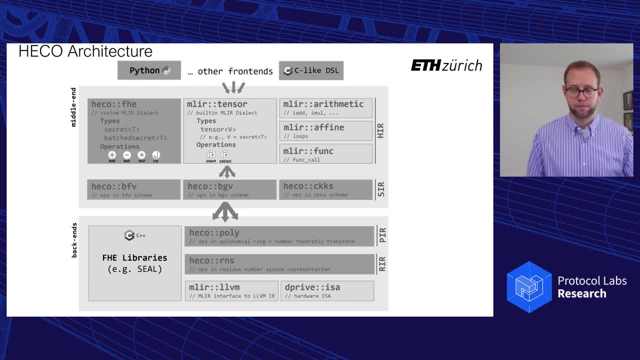 future it would get dispatched to a deep private system. So this is a very interesting way to try and accelerate it. I've already given you an example of what it looks like to take something from, let's say, BFB through to poly, but now I want to have a bit of a closer look at the high. 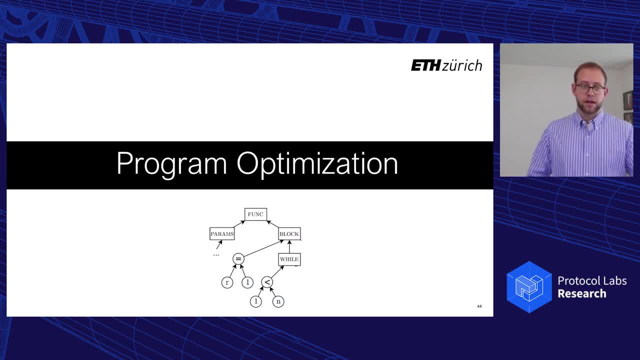 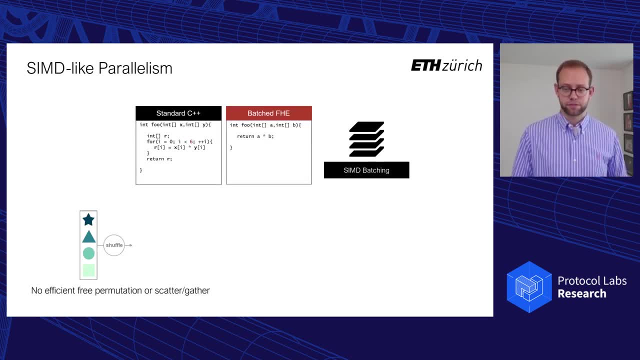 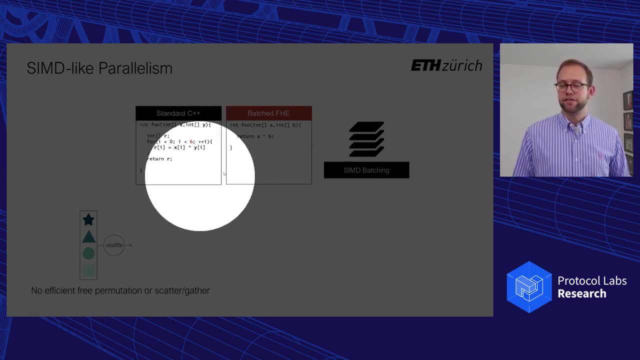 level transformations that I mentioned earlier, And in order to be able to do this, we need to have a quick recap of this SIMD-like parallelism, which I already mentioned. Obviously, it's amazing. It allows us to do things like replace many operations with a single SIMD operation. 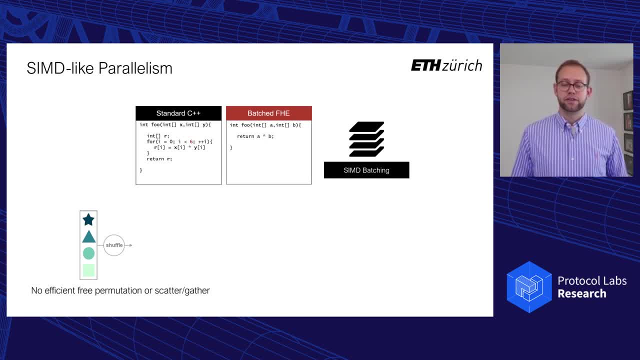 right, Great, But the catch is that it doesn't give us data movement. So in normal operations like ADX-512, which are very common, like server-sized vector operations, we can actually very efficiently permute or scatter-gather, and this is very heavily relied on in optimization. 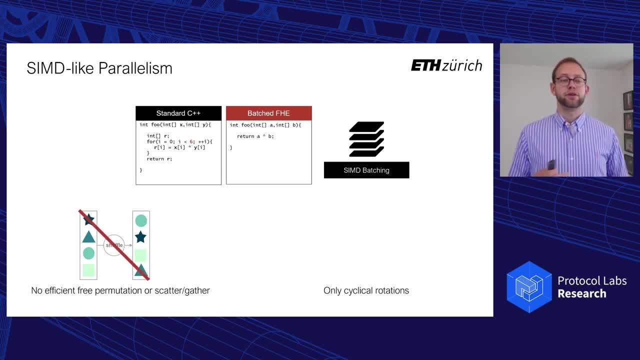 cyberting this In FHE. this is not an option. The only thing we can do in terms of data movement natively is cyclic rotation. So we can take a cybertext and we can add significant actual runtime costs, rotate it in a cyclical fashion And, because of this, restricted data movement. 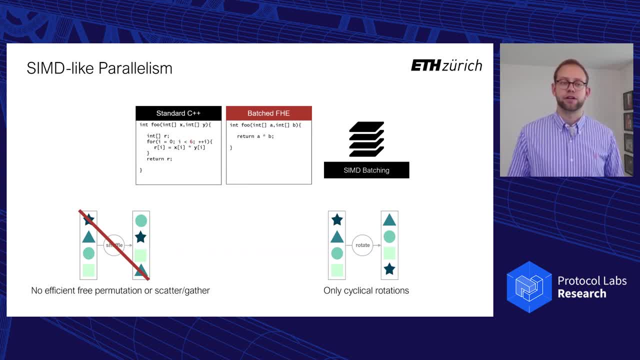 it doesn't really work the same way as computation paradigms that we see like ADX-512 or other vectorized products, And so really, how to use this to get latency improvements right? So how to accelerate a single instance of a program is very, very tricky and sometimes not very obvious. 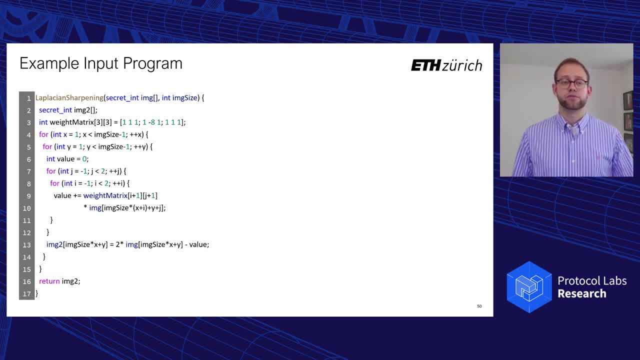 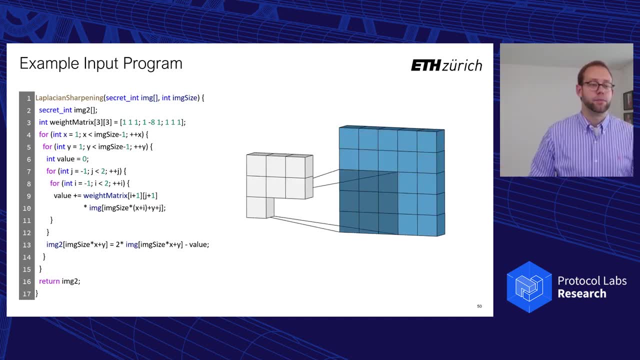 For example, this is a fairly simple program that computes a simple image sharpening right. It takes a kernel and it iterates it over the image And while it may not look like it, it is actually very FHE friendly. So currently it's in a very unfriendly form because we have all of these random accesses. 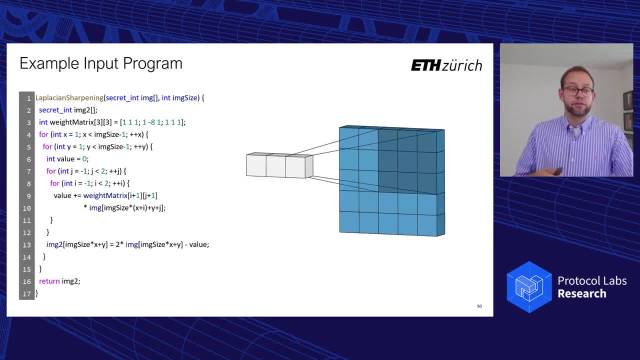 into these image pixels, which is very, very bad. FHE cannot do this sort of data movement or extraction of a single element from a vector efficiently, But this does actually have an efficient FHE implementation. The problem is that it's a rather dramatic transformation. 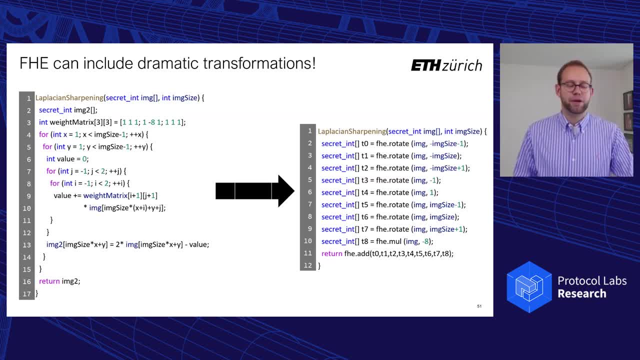 And I hope I'm not presuming here when I say that it's basically unrecognizable from the original program. For example, this inner loop here or this inner loop nest even has been turned into a single instruction in the FHE program. And these outer two loops, well they just completely. 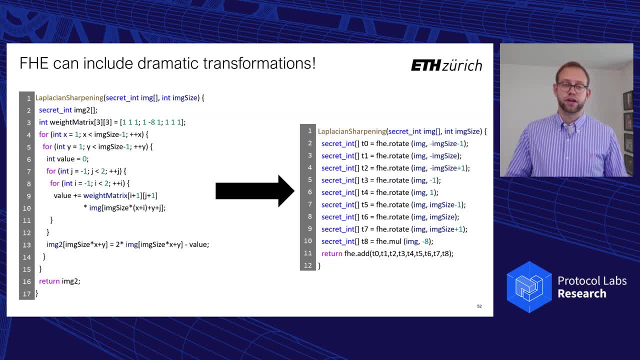 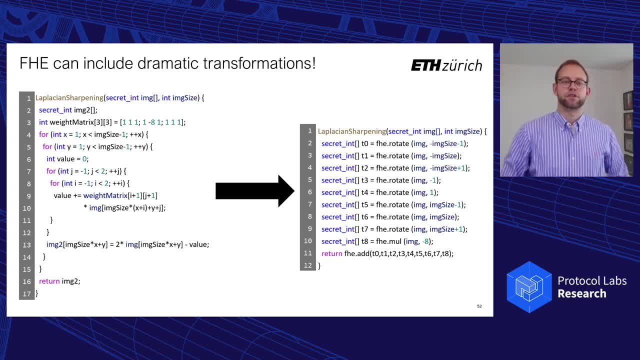 we're actually duplicating the image. So we're actually duplicating the image, So we're actually a few times rotating it appropriately and then jamming it through the kernel in one big SIMD operation at the end. And so this is an example of the kind of transformation that we need. 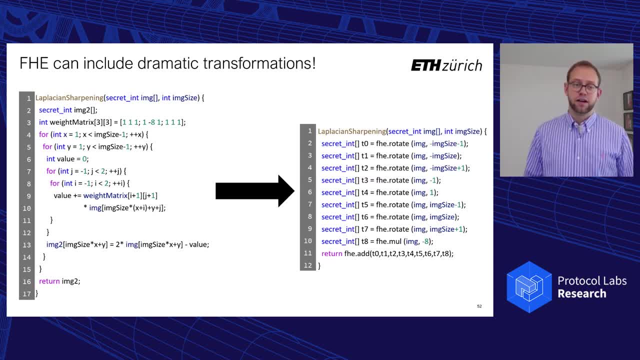 to do in order to get decent performance out of FHE, And it's also an example of how drastic these transformations can be. So it might be natural to resolve to things like synthesis or other sort of heavyweight tools to achieve this, But our goal here really was to do this. 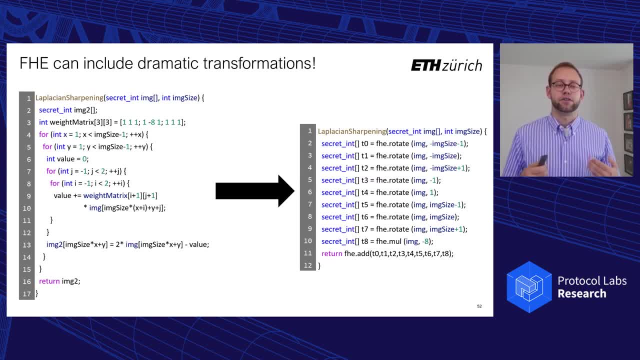 with simple and efficient translation boards that you can actually use in everyday development and programming. So in order to show you how HECO would tackle something like this, I'm going to drop to a slightly smaller and simpler example that will actually fit in the slides. 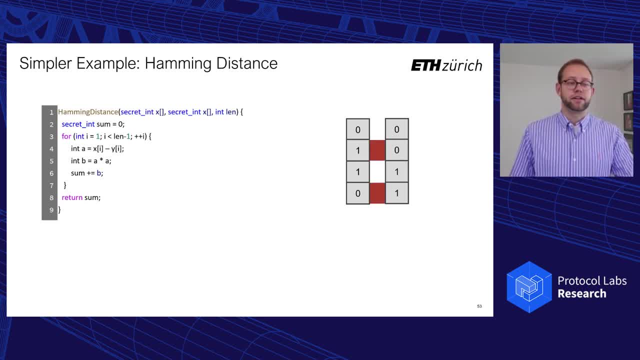 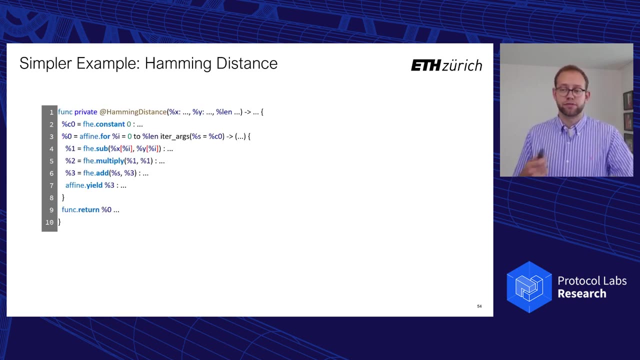 And that's the Hamming distance. Very simple task: Calculate how many positions of the vectors disagree, right? So the Hamming distance of this example is 2.. So this is like the C++ representation of the program. This is what it would look like in the high-level intermediate representation. 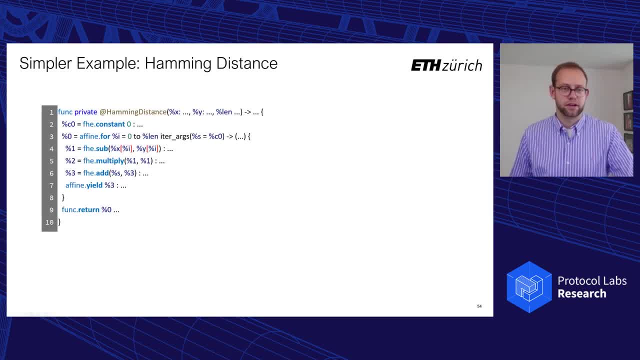 I've omitted all the typing information here, just because it gets very messy if we do that. So right now this has a lot of these random index accesses And, as I mentioned earlier, these are very bad for FHE. We can emulate them by rotations, multiplications, with mask and all. 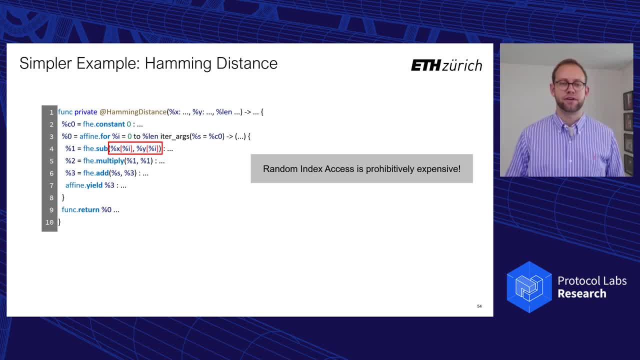 these kind of things, But basically they're just prohibitively expensive. At our point we actually show It's much more expensive than what we're used to. It's much more expensive than what we're used to, But basically they're just prohibitively expensive. At our point we actually show It's. 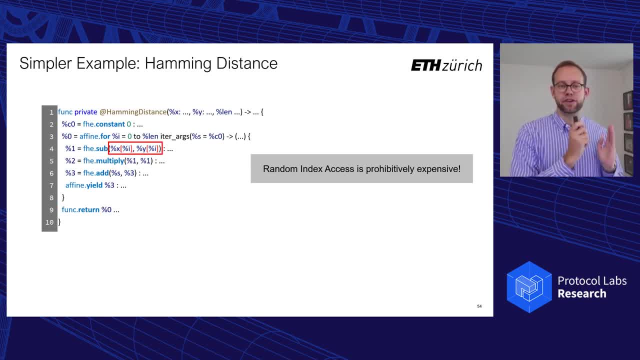 much better to not even bother with batching and put every data item into its own ciphertext, But that's not exactly a great solution, And so what we do is we want to try and minimize these operations. But before I can show you how we do that, I want to quickly. 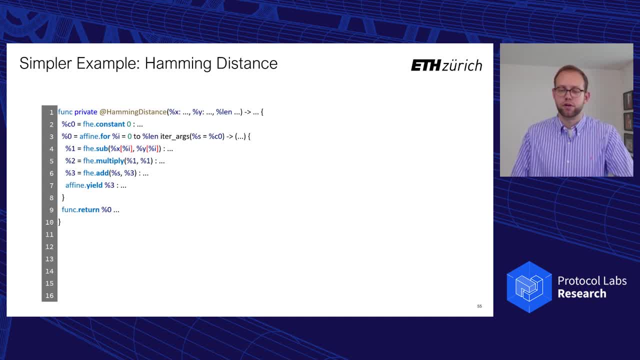 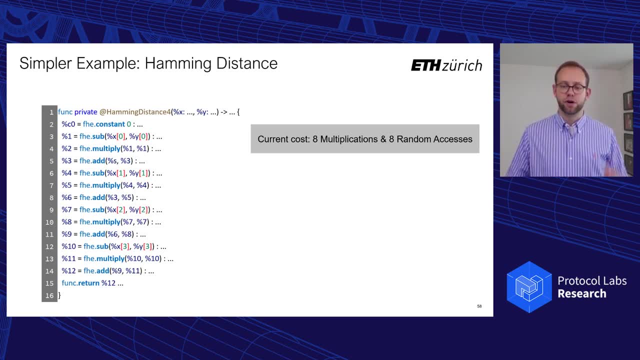 unroll this program just for exposition. It makes it a lot easier to follow along. So let's give this a few unrolls. There we go. Now we have a program It does the Hamming distance of size 4. Maybe not the most practical program, but it fits on the slide And it. 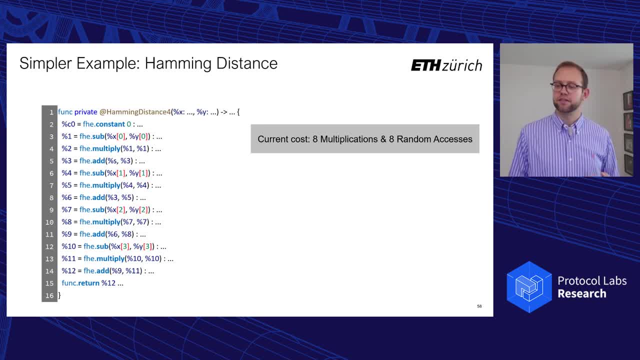 currently has a cost of eight index accesses and sorry, that should be four multiplications- And we want to make this better, And the first thing we're going to do is maybe not going to be super obvious why we're doing it, but we'll get back to it later, Because the first 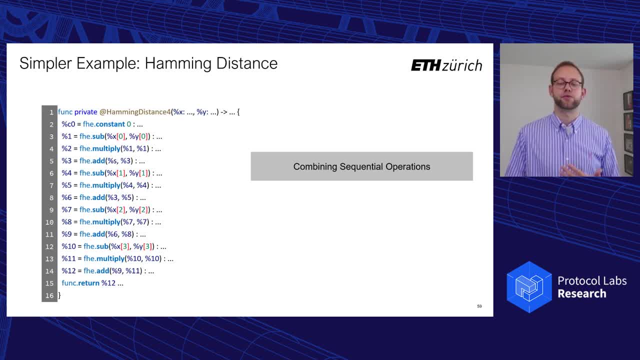 step in. what IKU does is it combines what we call sequential operations. For example, all of these additions here that we see they keep adding to the result right Like it's one series of additions And we can combine these into a single big addition operation. 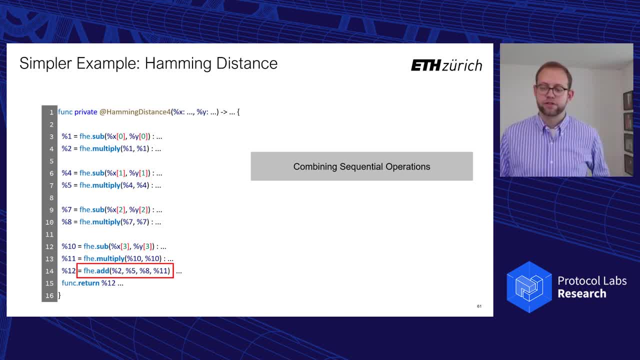 And we can obviously drop the plus zero because that's no longer relevant. And now, instead of having binary addition operations, we have n-ary addition, And this is actually quite important. later on, but for now, I just hope you will believe me that will become more. 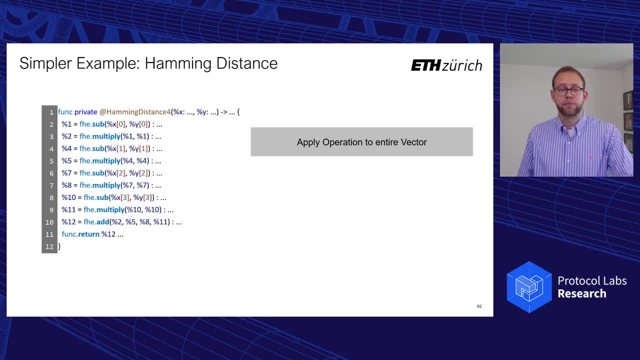 relevant. Okay, so this is the next step. It's much easier to see how this works. Okay, so this is the next step. It's much easier to see how this works. Okay, so this is the next step. It's much easier to see how this works. 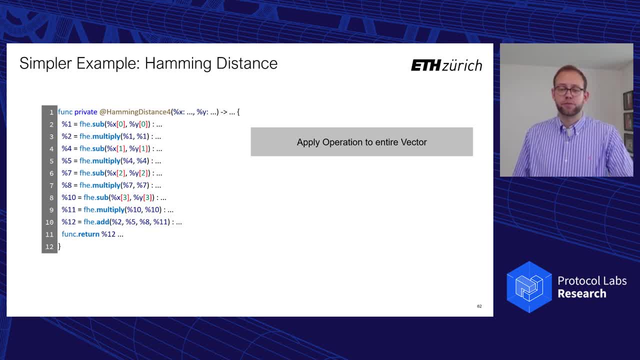 So we can see how this relates to batching, because what we do now is we look through the operations and we try to apply an operation instead of two individual vector elements to the entire vector. Well, that's great. We can get rid of all the other ones because 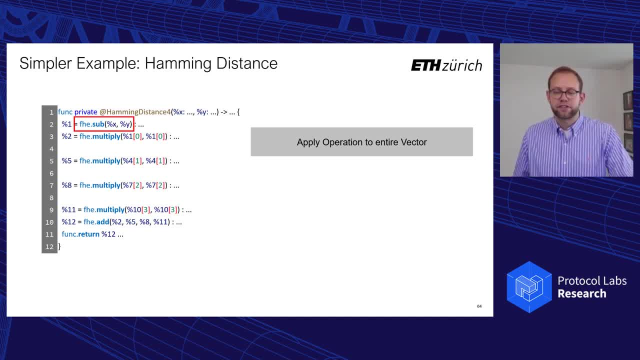 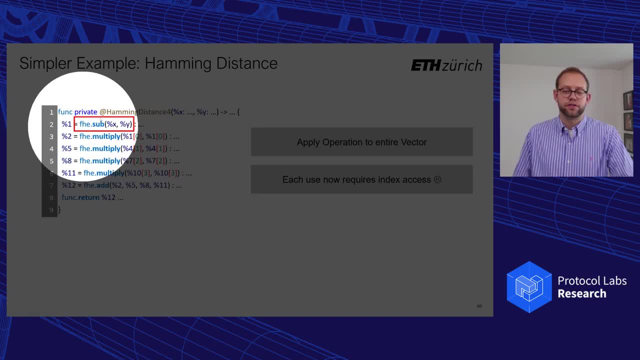 they're essentially being pre-computed by this operation, But the catch is that now what we need to do is we need to add an index access every time we use this result right? So instead of actually removing index accesses, we merely move them around in the program. 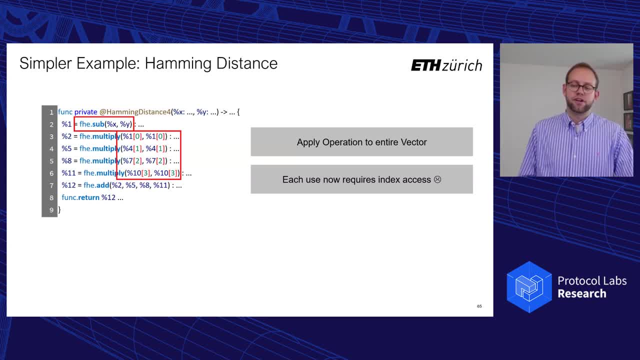 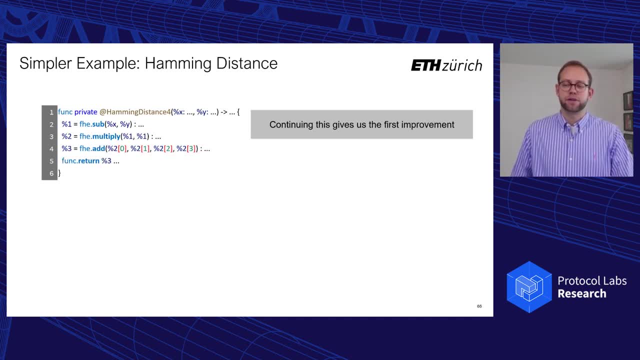 The good news is that if you do this replacement in a, let's say, clever way and you continue doing it, for example, doing it to the multiply here, then we're starting to see the first improvements. right Now, we only have four index accesses, rather than eight that we had. 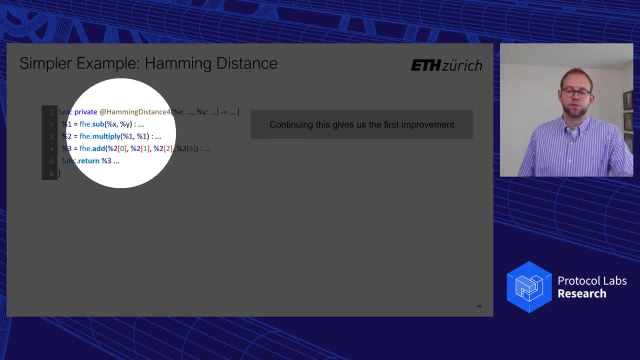 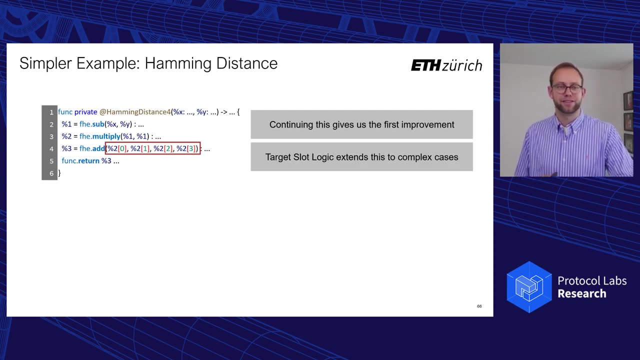 in the beginning, And we've also removed three of our four multiplies In practice in. like real-world programs, it takes a bit more than just hand-waving to make this always work, And so in the compiler we actually have a good amount of what we call target-slot logic. 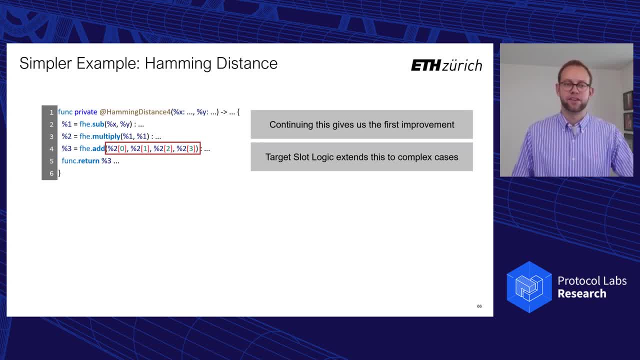 which decides how and where to vectorize these things so that this works out in as many cases as possible. Okay, So what have we done? We've made the program, I guess, not just 50, but actually more than 50% faster. That's really nice, And in the world of like Clang, that: 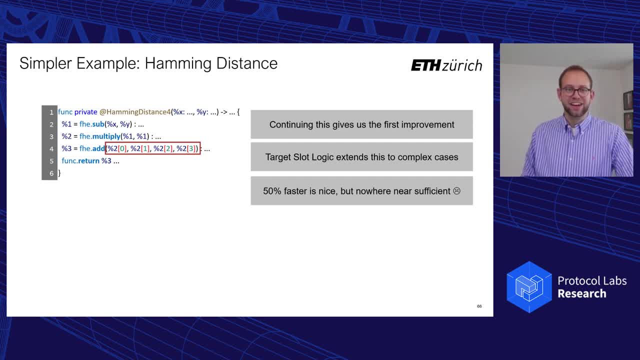 would be like a best paper award or whatever, But in the world of FHE that's just not even table stakes. 50% faster is no good, Yeah. So in your situation, in a world where the performance gap between Naive and Expert is, 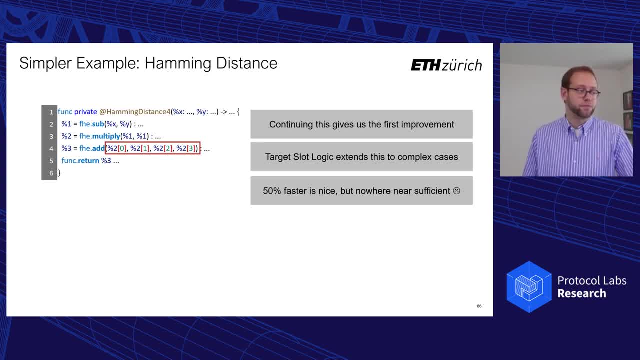 many orders of magnitudes in the worst case, And so I promised you we'd get back to this interesting addition operation, and that's what we're going to do now. First of all, we need to translate these index accesses here into rotations, So that means that we 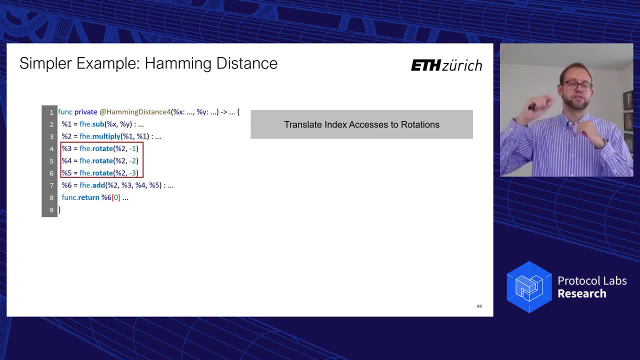 now, instead of fully emulating that, this is a scalar. we're just moving the value that we want to be on the same slot in each of the psychodecs that we need, And then we can then take the end of that and we can also take the second and the third slot that we have, So that rotations. obviously are a part of why index access is so expensive, but they're still cheaper than fully emulating index access. And then we can get rid of the last index access in this program by just saying: look, if we're trying to reach out a scalar, we'll just look. 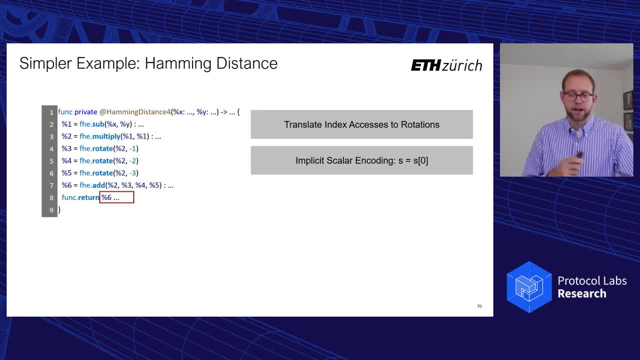 into the first slot of the zero slot of your psychodecs And that gets us to a program that now has no more index accesses, The single multiply. if you rotate, this is much more easy to go, And then we can take the second and the third slot and make sure that we have 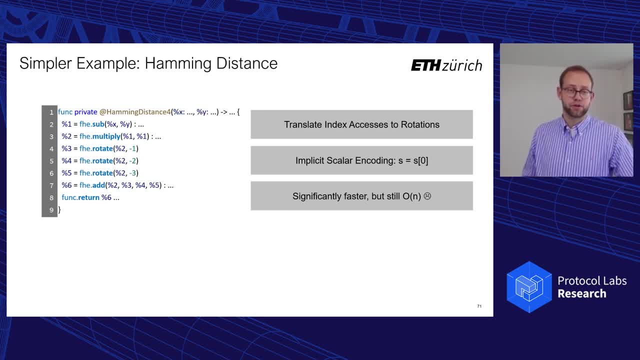 no more index accesses. So we just need to take the index access and just rotate them, And then we can take the second and the third slot and make sure that we have no more index accesses, And then much, much, much faster than the input program was. 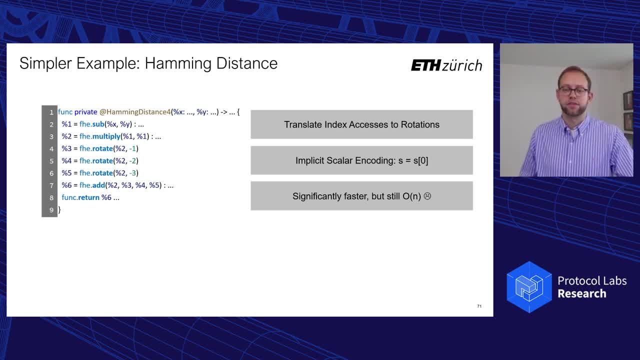 but most importantly, it's still linear, It's still O of N in the size of the input, And we can actually do significantly better here, And that's by exploiting that all of these inputs here have the same origin right, So all the things being added have the same. 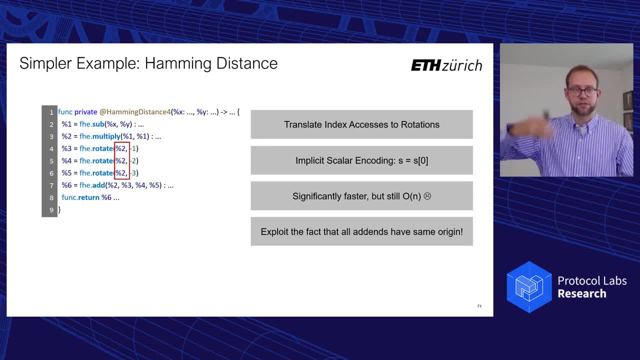 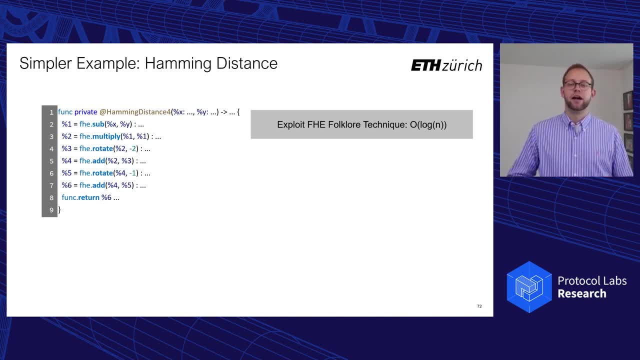 they originate from the same ciphertext, they're just different rotations of the same ciphertext. And here we are the first, as far as I know, to exploit, automate and sort of generic by this epigene folklore technique that is used to compute the sum of elements in a ciphertext. 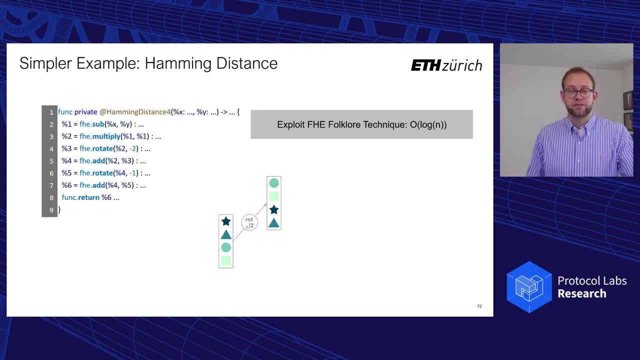 And the way we do this is fairly straightforward: We take a copy of the ciphertext, we rotate it by half, we add them back together to get the partial sum, and then we rinse and repeat this like a logarithmic number of steps until we have the sum in every slot. 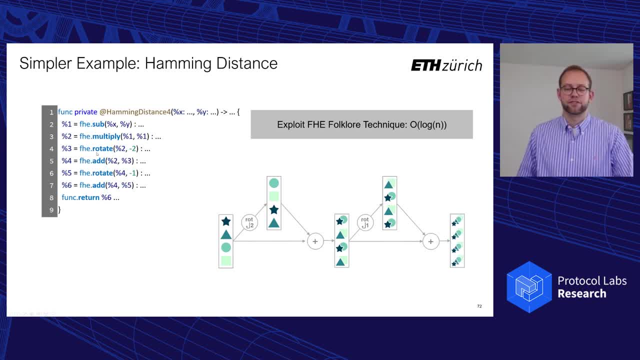 And obviously in the concrete example here, well, we went from three rotations to two rotations because at size four the difference isn't significant. but you can clearly see how for larger sizes, and in FHE we're talking 8,000 to 64k elements per ciphertext. 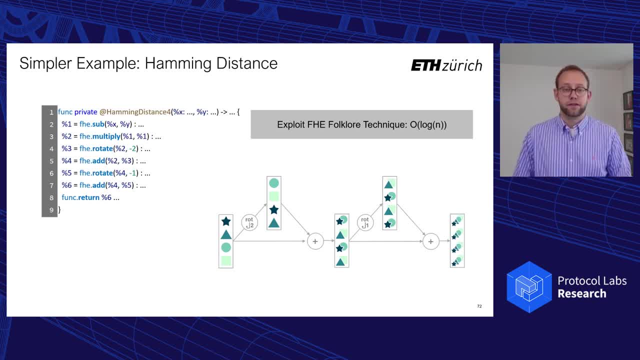 going from O of N to O of log N can make a significant difference in runtime, And I will have some evaluation results on this later. Okay, so this is sort of a toy walkthrough of what HECO does in terms of compilation When we zoom out a bit. I'm going to show you a little bit of what HECO does in terms of compilation When we zoom out a bit. 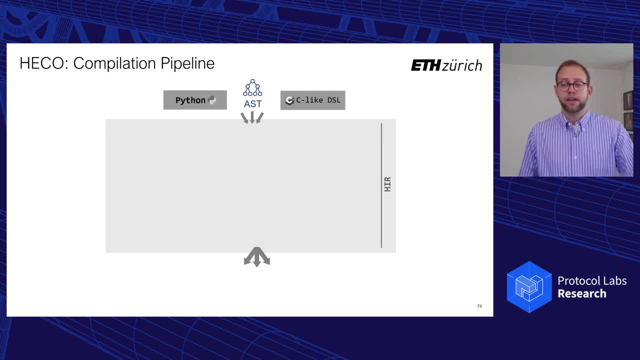 I'm going to show you a little bit of what HECO does in terms of compilation. The compilation pipeline looks like this: We take in an AST for the program from the front end. We then convert it into the SSA- high-level intermediate representation. 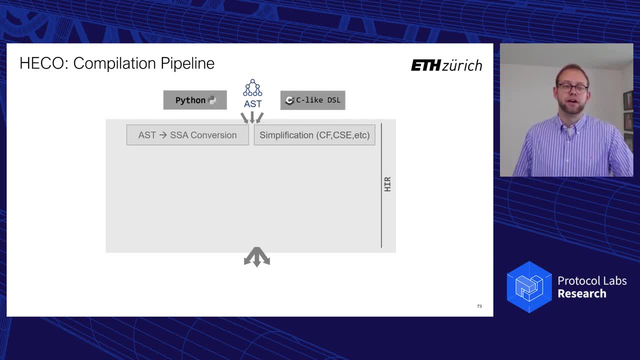 SSA here being single static assignment. It basically means we don't have variables that are overwritten again. It's a very standard form for compilers and makes it much easier to write optimizations. We also then apply a bunch of standard out-of-the-box simplifications. 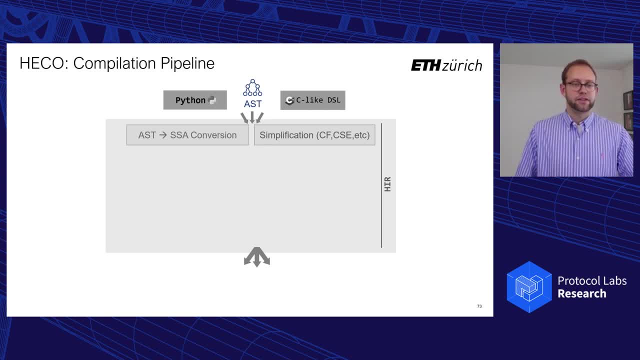 constant folding, common sub-expression elimination, sort of standard techniques that just help us get the problem size down a bit. Then we do what we call type separation, where we split the sort of vectors and tensors that appear in the program into the ones that are irrelevant. because they're operating on plaintext and stuff and the ones that we actually care about that operate on secret values, And that allows us to then do all of our optimizations only on the things that we should actually be optimizing, because it would not be good to apply FHE-style optimizations. 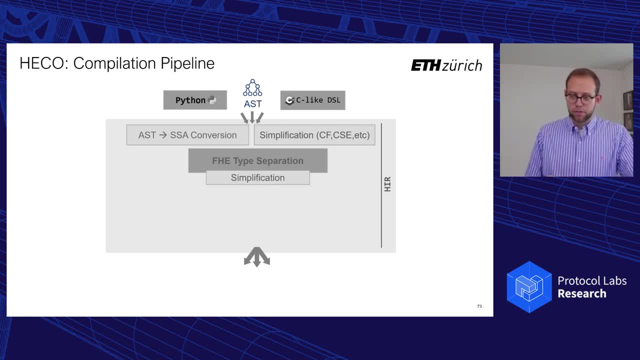 to standard sort of plaintext number crunching. After this we do another round of simplifications and then we do the vectorization parts, which is what I spent most of my time just sort of walking you through, Because vectorization powers could unlock more redundancies. 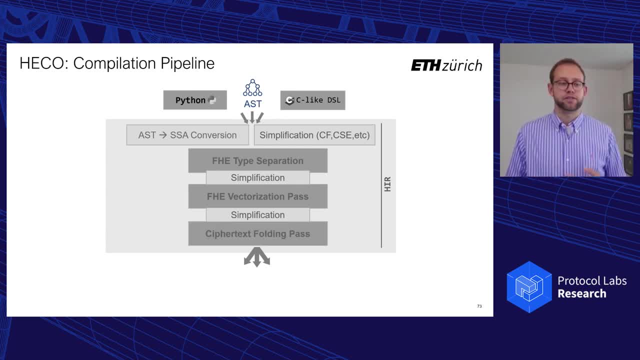 we do another set of simplification, before then finally doing the CipherDAX folding parse, which exploits this folklore technique that I just showed, And then from there, if you're sort of continuing this train, we go to the scheme-specific intermediate representation. 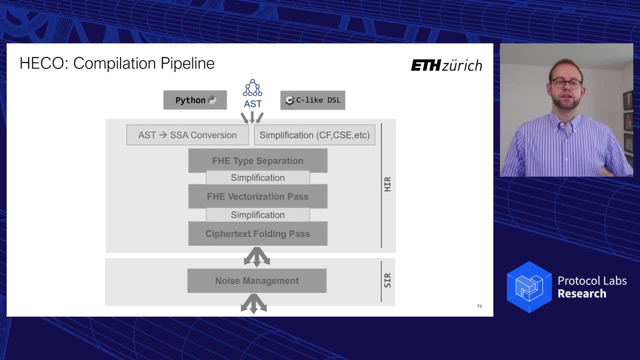 And that would be the point where we do what's called noise management, which is inserting CycloDex maintenance operations and all these other sort of slightly more technical intro to related aspect of the compilation. Okay, so that's what HECO does. 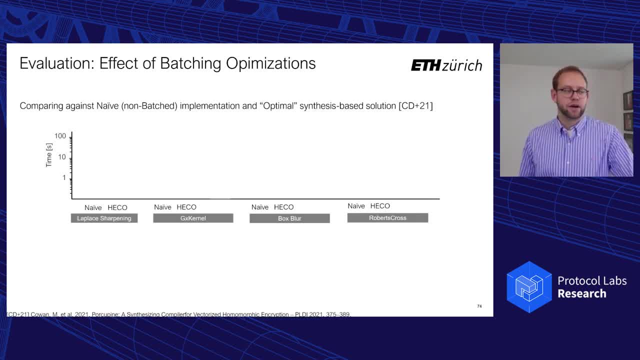 Well, how does it do? Well, if we look at some actual evaluation results of the optimization, we can see that when we compare HECO solutions against Naive non-veg solutions, we see about an order of magnitude speed up. 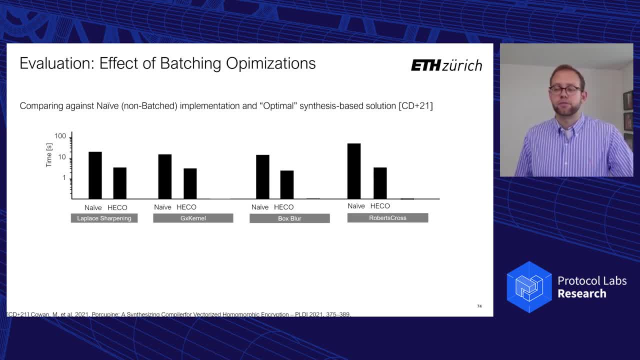 So that's a log axis right, And we see that in pretty much all of the cases we get at least an order of magnitude speed up, And that's great in itself, I think. as a result, But in order to show that we're not just sort of doing some speed up, but that we're actually finding sort of what the experts would have written, we're also comparing, where possible, to a tool called Porcupine. 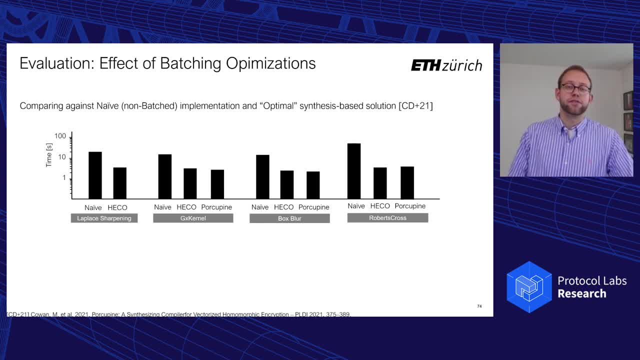 So Porcupine is also an FHC compiler, but it's a synthesis-based tool, So it really only works for sort of toy sizes And it takes even then. It takes up to like 20 plus minutes and sometimes just absolutely fails. 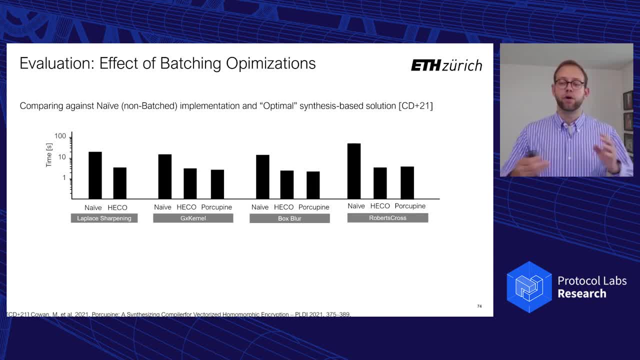 But where we could evaluate it, we could show that HECO and Porcupine actually produce essentially the same output. There are some situations where Porcupine is ever so slightly better than our tool, but it's basically within the margin of error on this kind of scale. 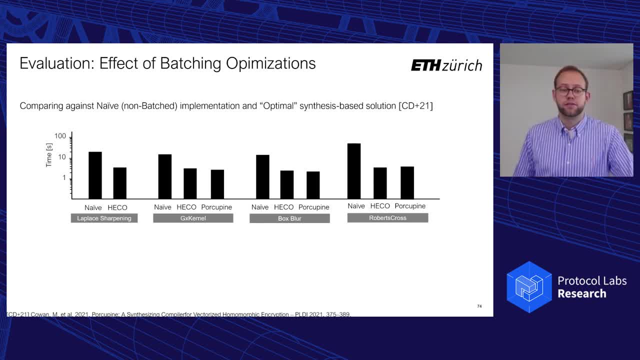 And so what we're showing with HECO is that you can, in fact, achieve near expert batching solutions for a lot of different programs, The same way that the synthesis-based solutions do, The same way that the synthesis-based tools have been doing it, but actually do it in less than a second of compile time, making it actual practical to give it to non-expert developers and ask them to integrate this tool into their sort of- you know, develop compile debug cycle. 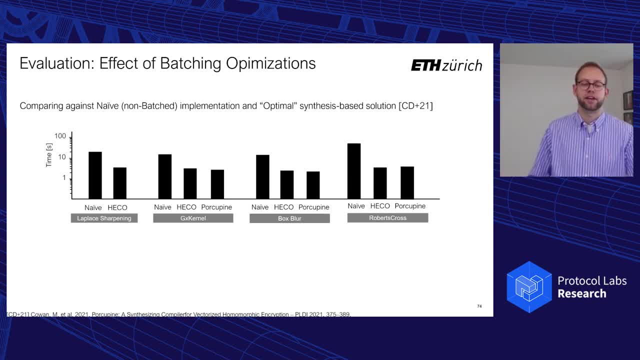 Because obviously you cannot go wait for a 20-minute synthesis compilation every time you want to do something. Of course, HECO also scales to more real-world example sizes And in the paper which is currently on submission- but we have a preprint of an archive- 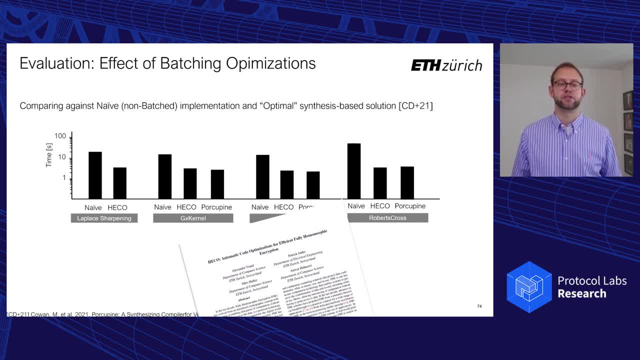 You can see more about how HECO scales to actual larger sort of real-world size problem instances. This is me nearly finished, but I want to do one quick diversion before I conclude, which is that I want to briefly talk about FHD standardization. 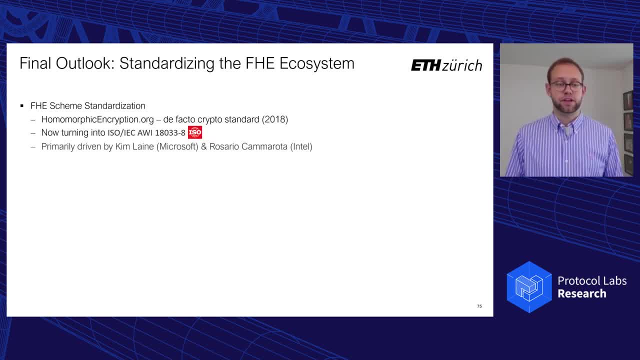 And so maybe not in the way you're thinking about, which is the scheme standardization. This is actually going amazingly well. For several years now, we've had a great de facto community standard which specifies sort of what levels of security are considered acceptable, what parameter sets are considered safe, and so on. 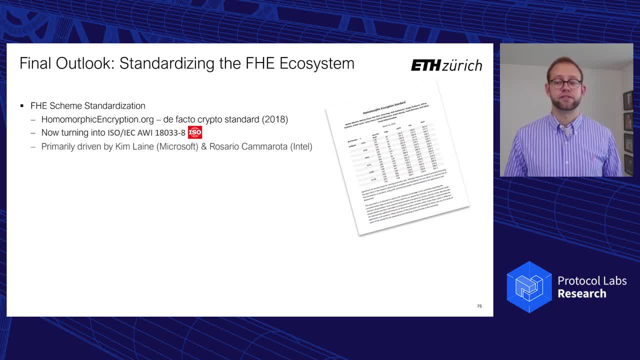 And, as a result of this, being very, very stable over the last few years, this is now being turned into an official ISO standard And it's being driven by Microsoft and Intel primarily right now, but obviously, as an ISO standard, it has a huge community around it now working on it. 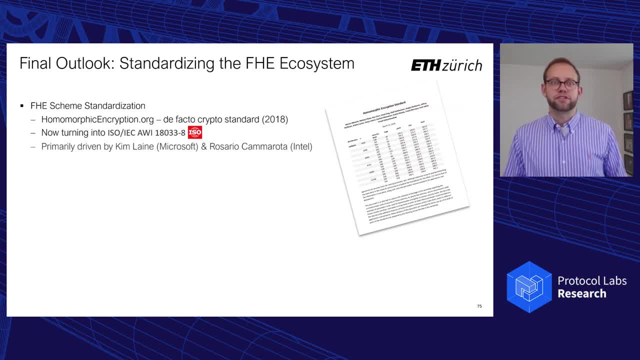 And I'm very optimistic that, you know, within the sometimes glacial pace of an ISO program, this will come out fairly soon And then we'll actually have a very fixed and nice description of all the standard schemes. What we don't currently have, and what I obviously, as a compiler person, care about much more, is standardization in terms of intermediate representations. 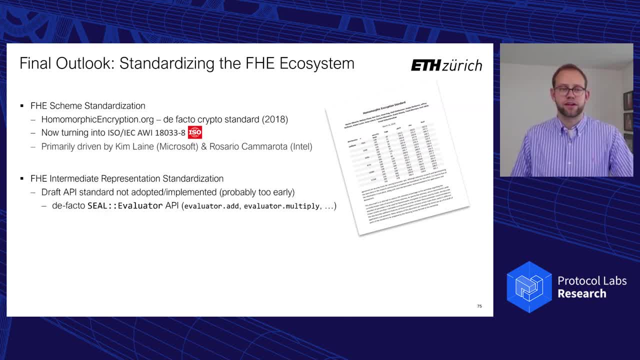 We did have this draft API that came out around the same time as the original community standard for the schemes, But I think it was just a bit too early at that point, So what we ended up with instead is just a de facto conceptual API. 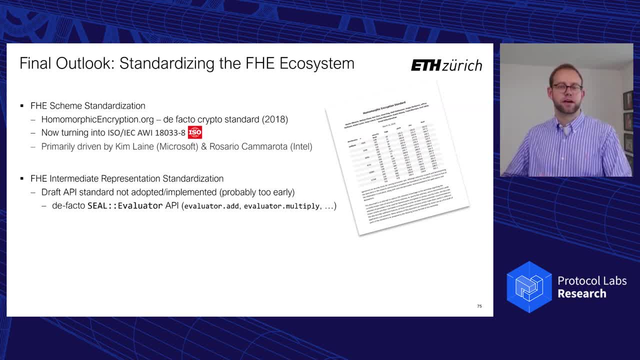 For example, SEAL has an evaluator operator. It's a project that then offers add, multiply, et cetera, functions corresponding to the scheme operations, And pretty much all the other libraries follow a similar pattern. The problem is that, well, first of all they're different, but that's just an engineering question. but also conceptually it's not quite sufficient to really think about and argue about.